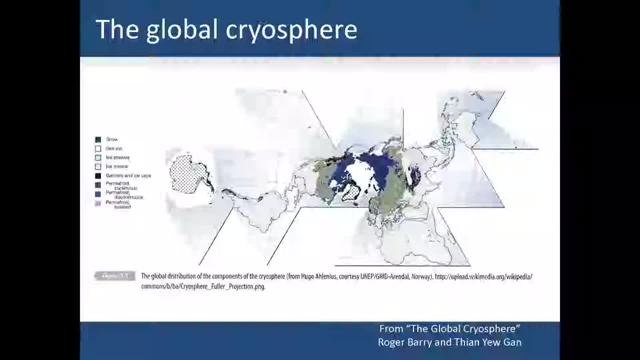 The blue there is of the permafrost regions of Northern Canada and Russia, And the green of the- Yeah, perennial snowbacks, the seasonal snowbacks, which of course come and go with the seasons. So I'll be talking about all these various aspects. 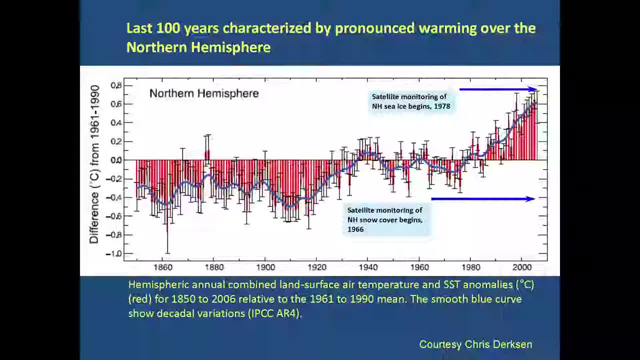 There we are, But of course the thing that is driving the changes in snow and ice are the rising temperatures worldwide. You're very familiar with these sorts of graphs. In the last hundred years, a marked global warming, And the snow and ice areas of the world are the ones which are suffering most or most responding to those changes in temperature. 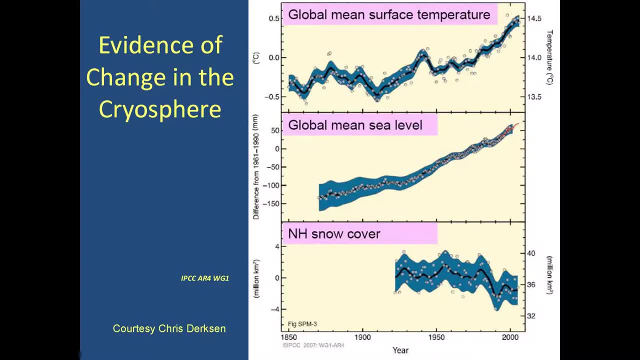 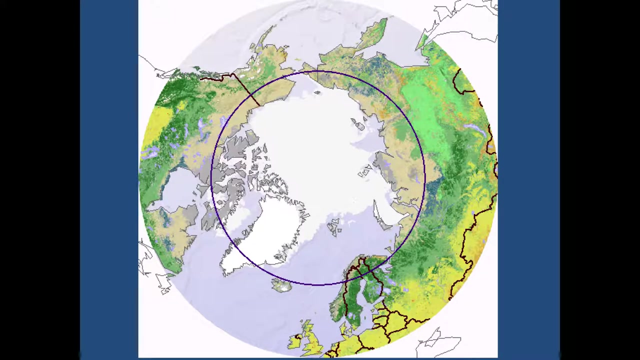 You'll see that not only have- Not only have mean surface temperatures gone up. That is associated with a rise in global sea level And Northern Hemisphere snow cover you can see there has been going down over the last few decades. Well, let's start up in the Arctic and consider first of all sea ice extent. 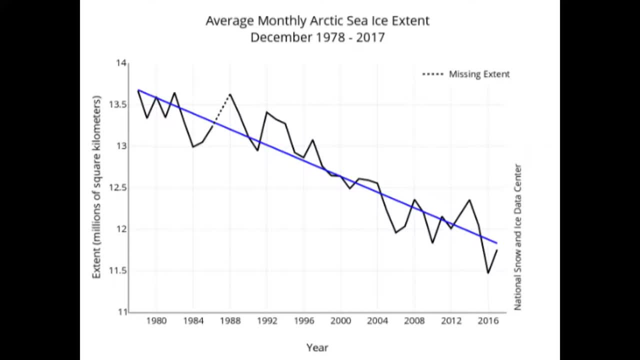 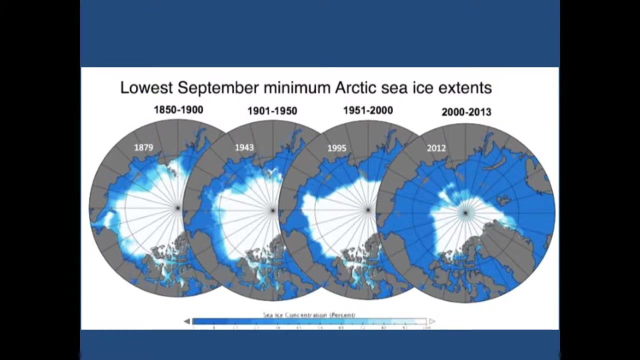 I think you're all familiar with these sorts of graphs Over the last 40 years or so And before that, if you project backwards- a general decline in sea ice cover- And in this graphic, of course, a hundred years ago, that was a projection backwards in time. 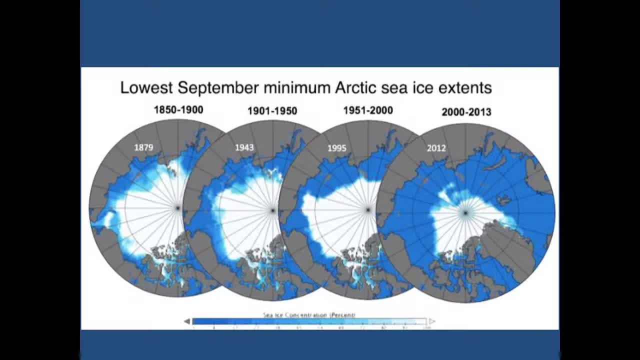 But obviously a decrease in the extent of sea ice in the Arctic, Leading to- And not only the aerial extent, of course, but the thickness of the ice itself is diminishing too, Allowing all sorts of things to happen in the Arctic Ocean. 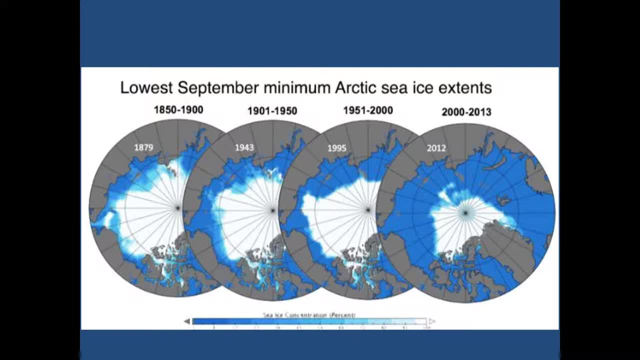 Including, as you know, cruises through the Northwest Passage, now possible And, in fact, in fact happening. And one of the places where I first studied was Svalbard Way, north of Norway. That was my first expedition as an undergraduate student back in 1963. 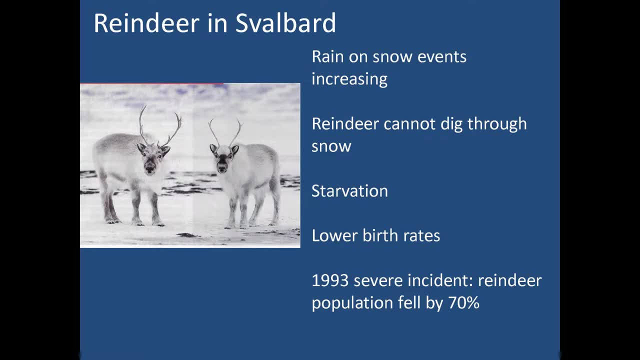 And just last week in The Economist there was a really interesting article on reindeer in Svalbard And how they, the reindeer herds, are suffering Because of warmer winters And the suffering is induced by rainfall events happening during winter. 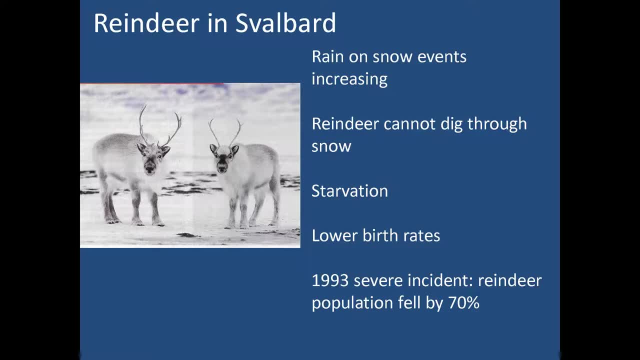 When it's supposed to be really cold and there's supposed to be no rain, And that rain percolates through the snowpack and then refreezes into ice layers, Leading to starvation of the reindeer Because they cannot dig through the snow to get to the vegetation underneath. 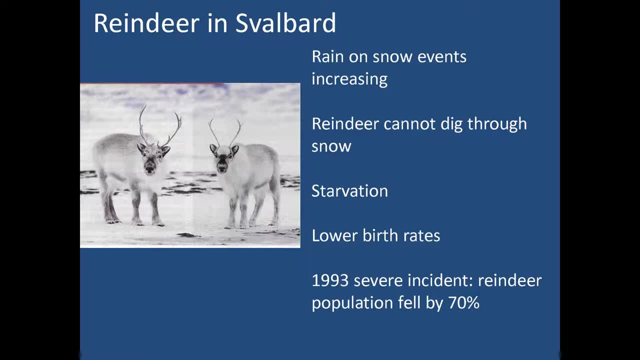 And this has led to lower birth rates. And the question is: are reindeer at a sort of tipping point? What if you had two winters in a row when there was a lot of rainfall and snow events? Because in 1993 there was one very severe incident. 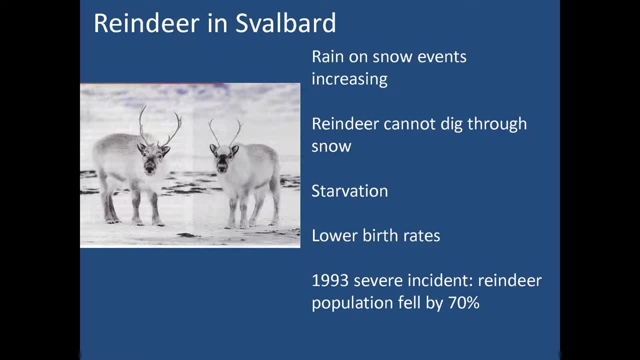 And the reindeer population fell by about 70% Just as a result of that. So here is an interesting ecological change associated with the changing cryospheric conditions, And in fact it's not only reindeer but it's arctic foxes and it's ptarmigan and other creatures that have been affected. 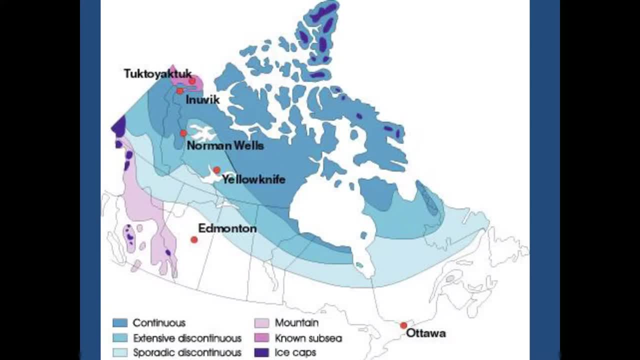 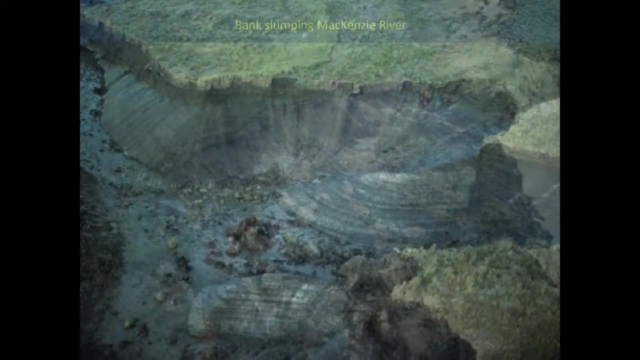 Thelma Frost, of course, as you know, is present in either continuous or discontinuous form In much of northern Canada, And the Thelma Frost is slowly retreating northwards. Those maps have to be redrawn And you're probably familiar with these sorts of photographs. 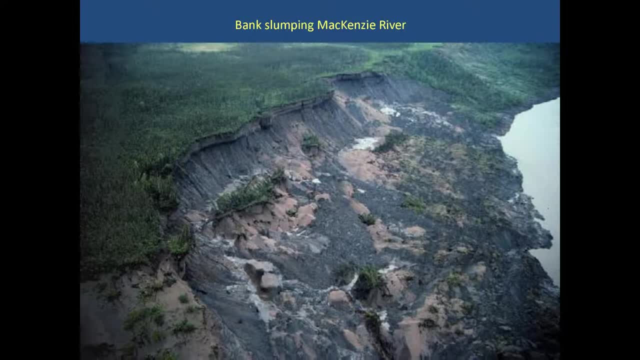 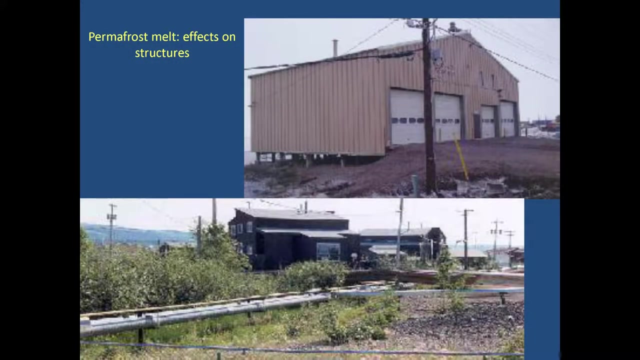 Of the slumping of the sides of the rivers and so on, And presumably having quite an effect on central Canada. Quite an effect on sediment transport in rivers affected. This is on the Mackenzie Effects too on human settlements. Structures are falling over, tilting over as a result of Thelma Frost thawing. 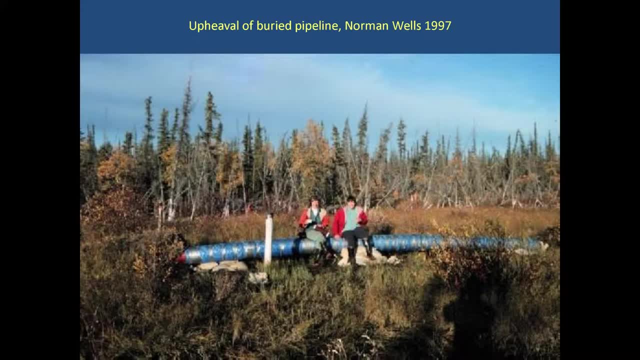 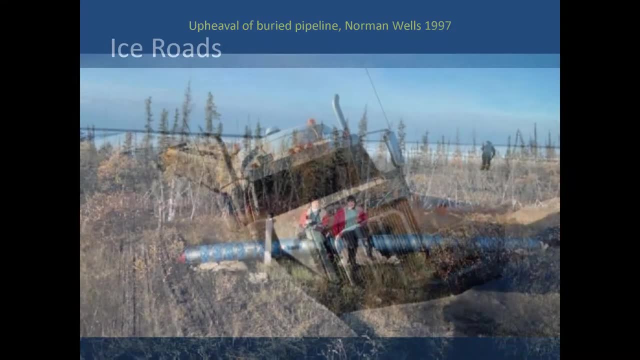 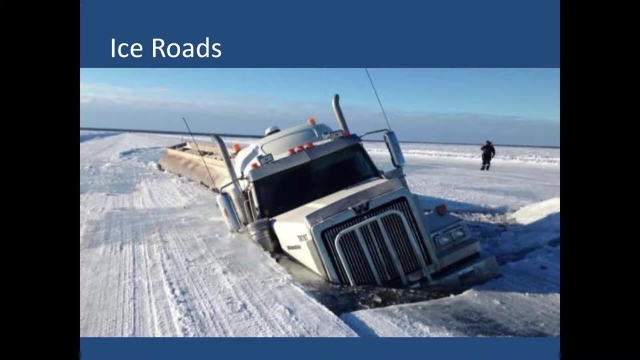 And there are many examples of this. for example is a pipeline which has been buckled up Because of the changes in the Thelma Frost, And we all hear about these ice roads in winter, Very important for northern communities. The roads are simply not there in summer. 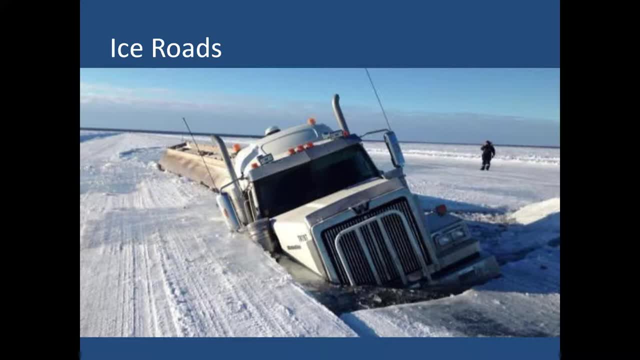 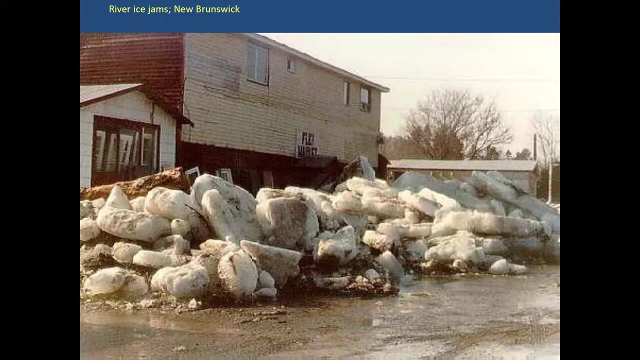 And winter transport is essential for many distant northern communities And because winter is becoming shorter and ice is becoming thinner on lakes and rivers, Then you get situations like this, And this is definitely affecting many of the remote communities in northern Canada: Ice jams. 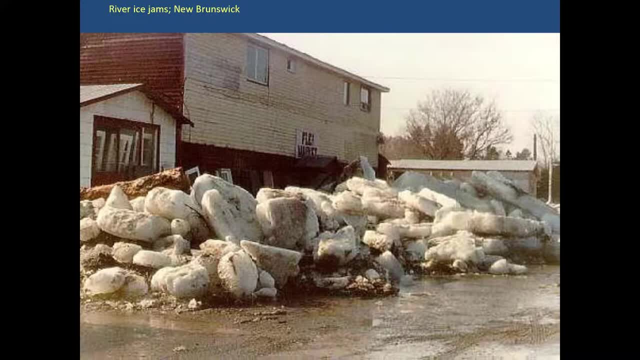 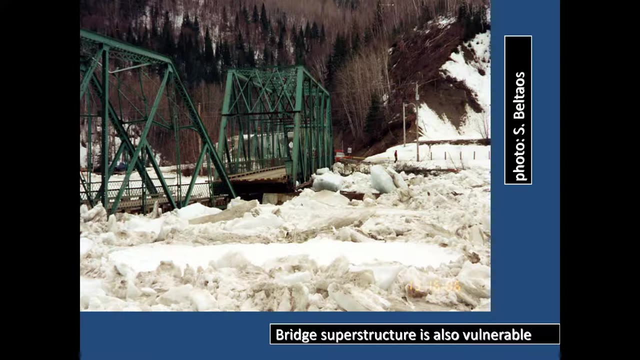 I don't know an awful lot about whether ice jams are getting worse or not. I presume that if the ice is thinner and not so much of it, there won't be so many ice jams, But I'm not exactly sure of that, And this is a photo from a colleague of ours, Spiros Peltaios. 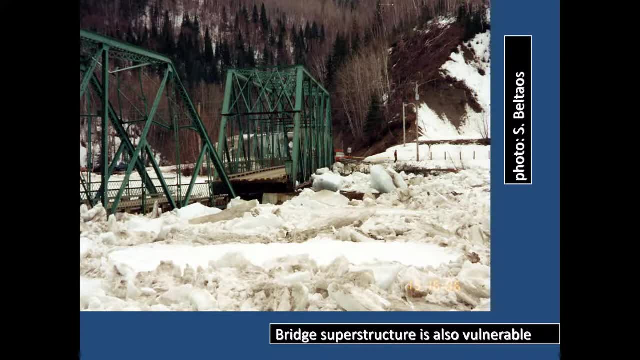 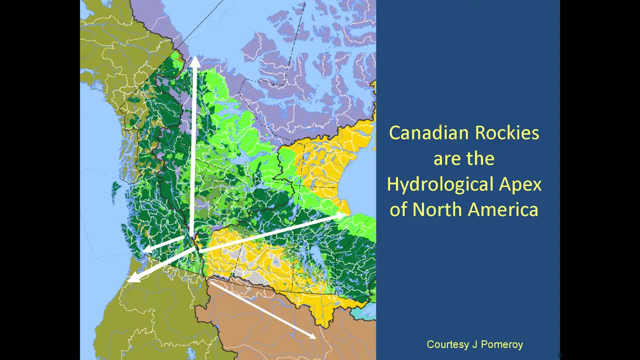 And you can see the effects of ice on structures And, as I say, I'm not really sure what changes in ice I mean, how they're being affected. Well, let's go to a happy hunting ground of mine And of my good friend Scott Moreau, sitting here in the audience. 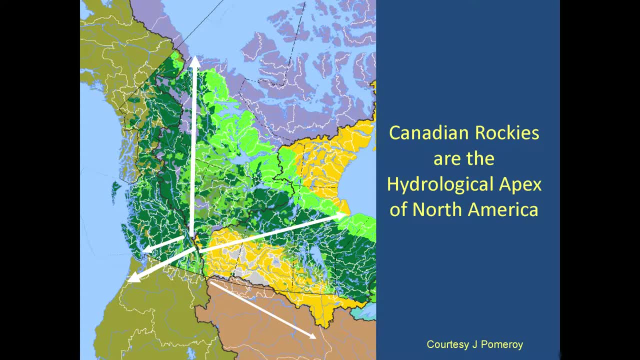 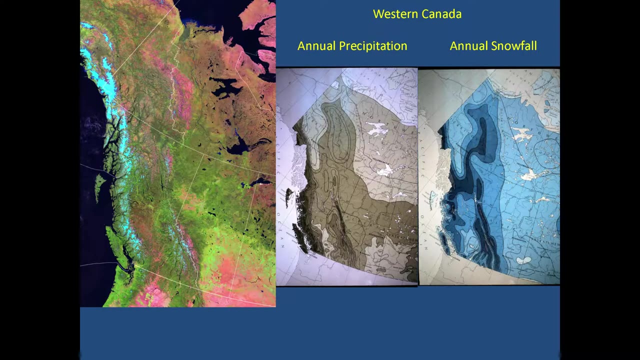 And of one of my PhD students sitting just in front of her. Let's go to the Rocky Mountains and have a look at some of the things happening there. On the left, the extent of glaciers. On the right, the precipitation amounts associated with those glaciers. 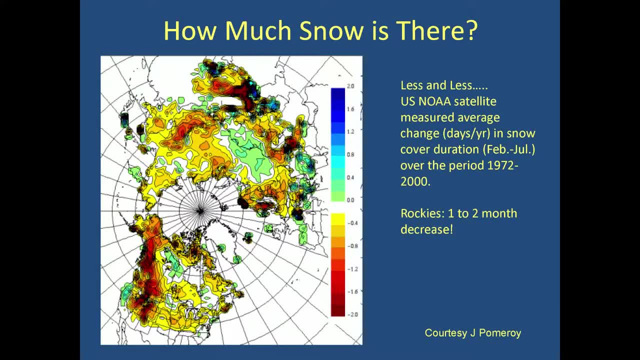 But this is a really interesting picture of how snow cover is changing in the mountains. The duration of snow cover Winters are in fact getting shorter, And here you see- Oh sorry, The Rocky Mountains. In fact, the snow cover is something like two months shorter in the Rocky Mountains now than it was 40 or 50 years ago. 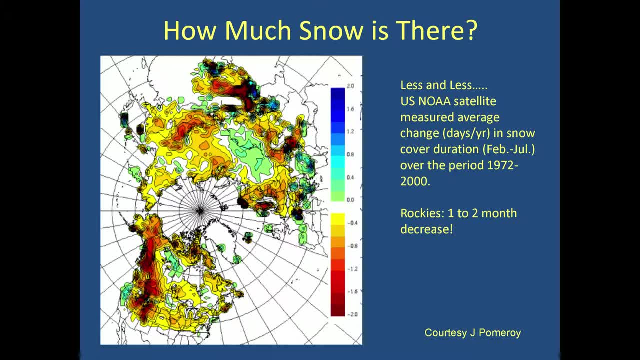 And this, of course, is having an effect on when the snow melts, How much snow is to melt, And when the snow does melt, It leads to changes in the regime of the rivers, Which, arguably, are important downstream for the use of the water. 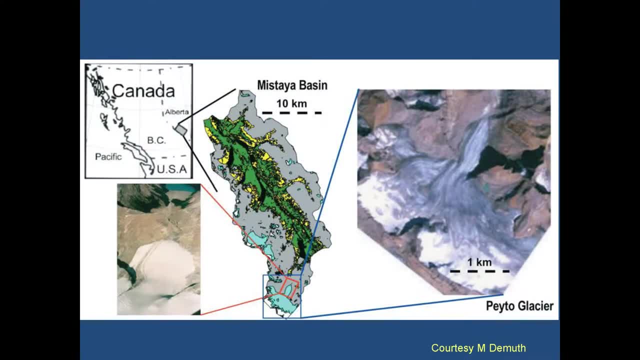 Well, we're going to the Mistea Basin Which, if you've traveled from Banff to Jasper on that glacier highway, you will have gone through the Mistea Basin. It's part of the North Saskatchewan River Basin And it's about 200 square kilometers in size. 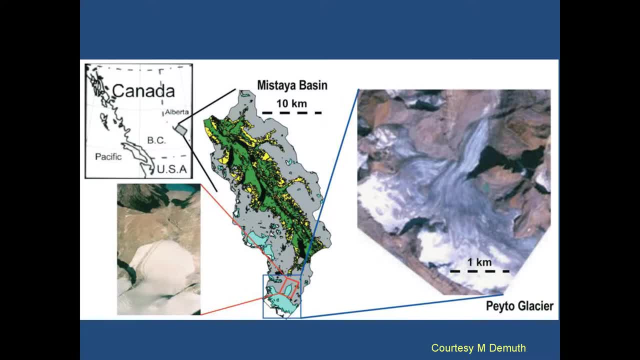 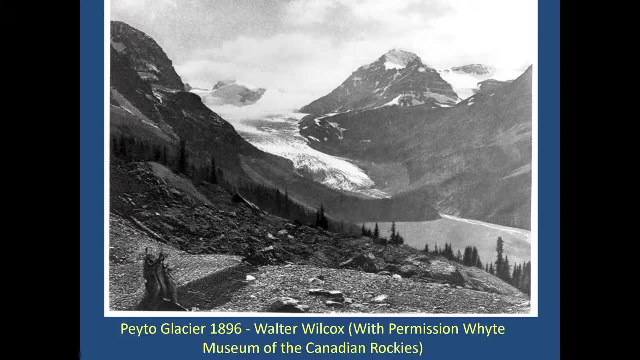 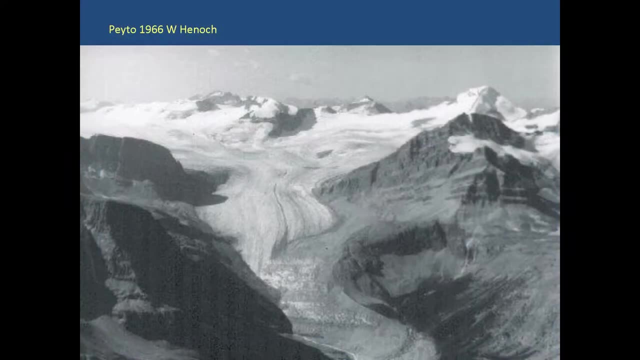 And within the basin is the Pato Glacier, And since 1896, this is the oldest photo that we have, I believe, on file- The glacier has retreated. This is its position in 1966. Just before I started my work there. 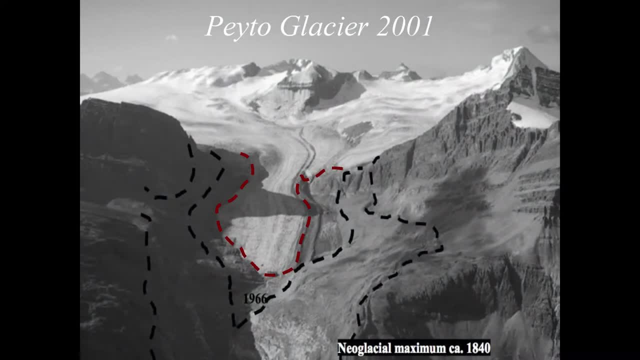 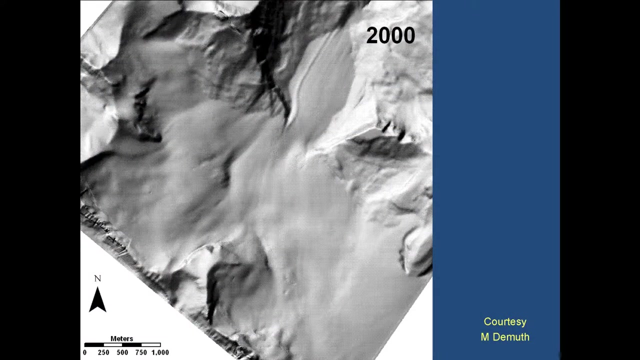 And you can see now in 2001,, that red line is where it had retreated to then, And since then it's gone back very much further. This is again in about the year 2000.. And here actually this is going from 2000 to 2007.. 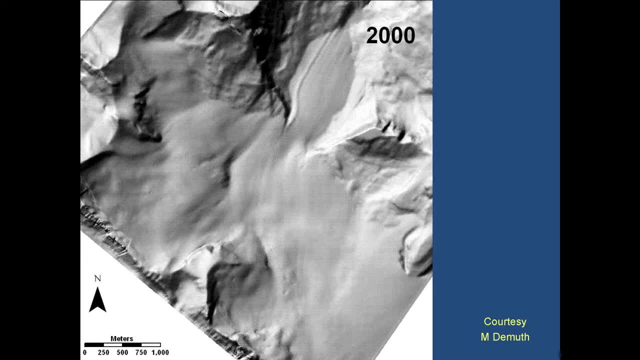 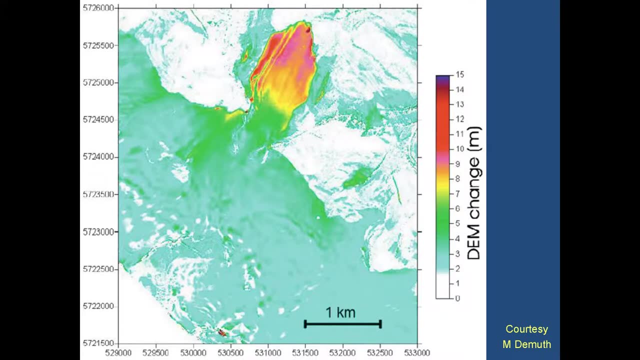 A series of images From LiDAR surveys And you can see that the glacier is getting smaller And it's that lower part of the glacier which has retreated and disappeared to such a great extent. Well, now that is ice coming out of semi-permanent storage. 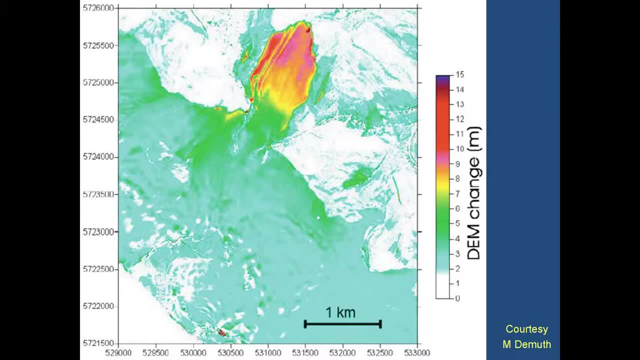 You have seasonal storage, Seasonal snowfall, Which then more or less disappears during the summer. But on top of that snowmelt and on top of the rainfall which occurs during summer, there is an addition of glacier ice coming out of permanent storage. 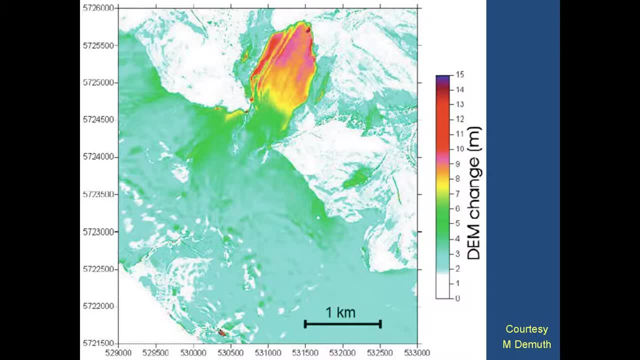 And that is important for the regime of the rivers. And you can easily appreciate that the more the glaciers disappear, the less water is coming from them, Because water is coming from that source, From that water source And in areas downstream where water is extremely valuable. 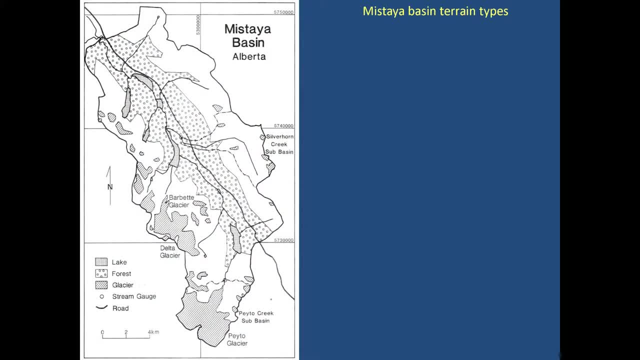 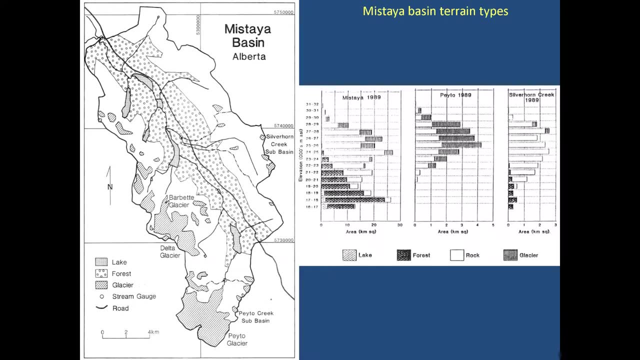 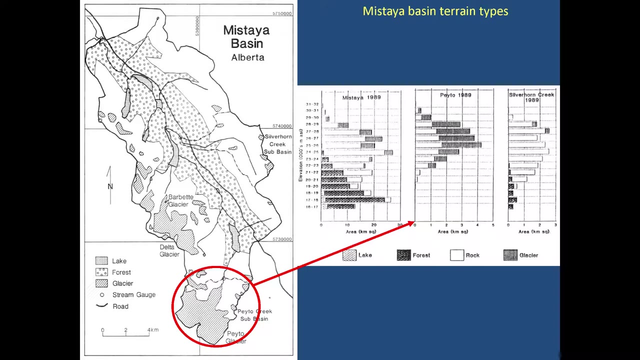 then that's very important. Just to show you the effect that glaciers have on stream flow, we can take the Pato Basin which I showed you just a moment ago, Highly glacier covered- Something like 60% glacier covered- In contrast to a very similar sized basin just across the way. 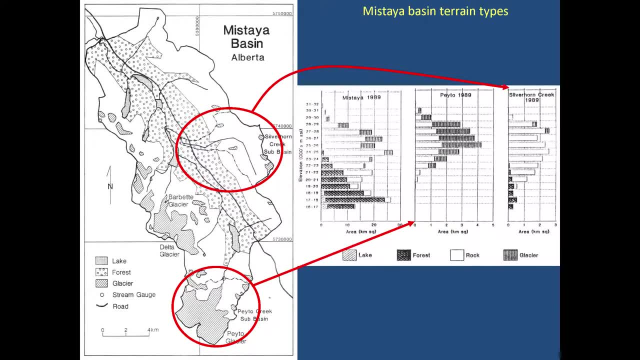 And Pato is north and east facing. It's in shadow. On the other side of the valley, the slopes are south and west facing. They're in sunshine, In simple terms, And so the glaciers are packed on the west side of the valley. 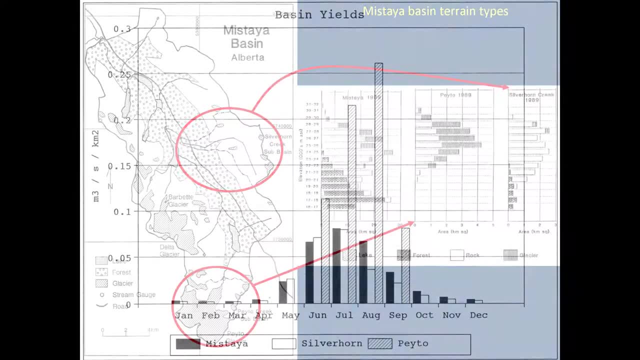 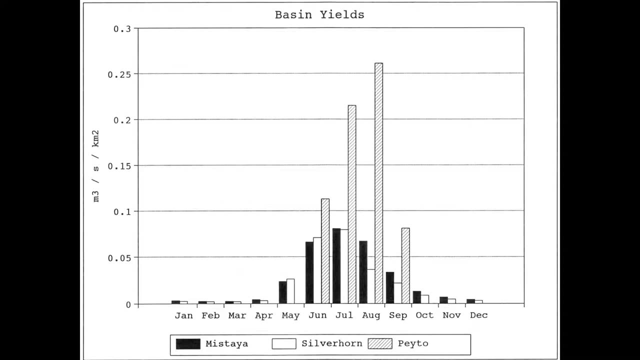 And the result is in the discharge Pato you can see that striped line- far higher discharge- because the glacier is contributing a great deal of water, Water coming out of semi-permanent storage- And you can see that it comes fairly late in the summer, with a peak in August. 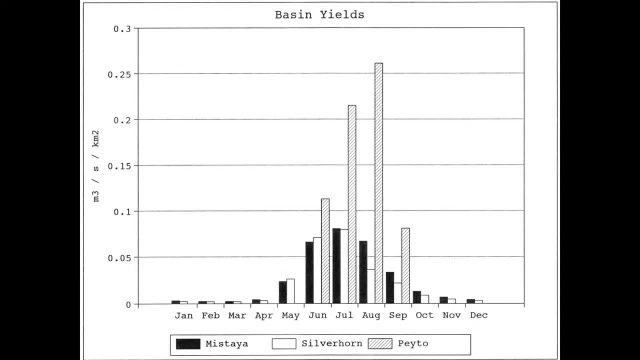 Whereas the Silverhorn Creek, the basin on the other side, on the sunny side, with almost no glaciers in this- Sorry- The open area. here You can see that the highest flows are in June and July, Snow melt peaks And there's no influence of glacier melt. 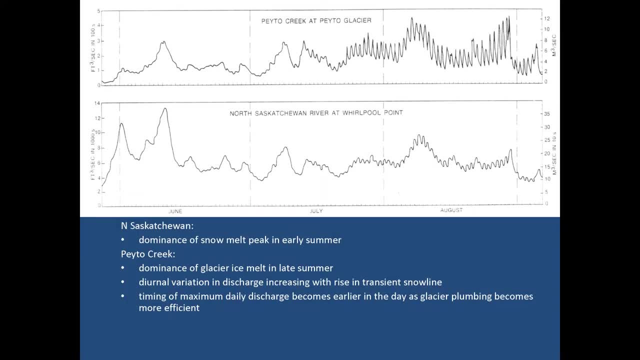 Here's just another example: Pato Creek at the top for one particular year And compared to the North Saskatchewan much further down, with much less glacier cover, The Pato has a snow melt peak here, But the highest flows are late in the summer, in August. 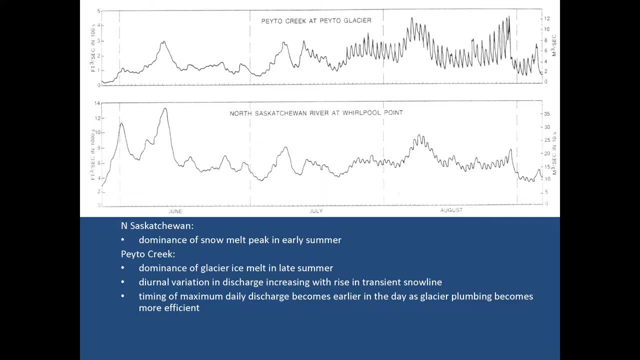 Whereas the North Saskatchewan, with a far smaller glacier cover, has a big snow melt peak, And that's the dominant peak. Nothing else compares to it. You'll see these up and downs here. Those are diurnal fluctuations. The glacier melts during the daytime. 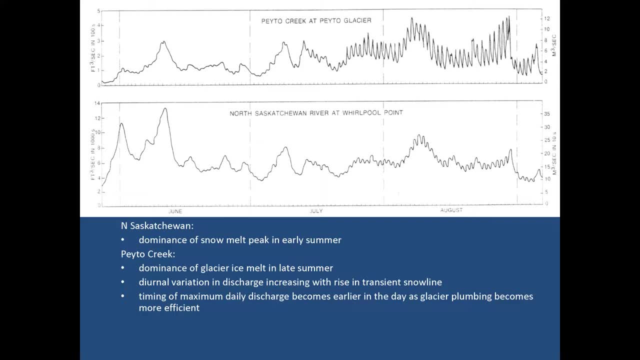 And it sort of shuts down overnight And this is reflected in the discharge. If you want to cross a glacier-fed stream, you cross it really early in the morning, Otherwise you may be washed away later And those diurnal fluctuations are really really prominent. 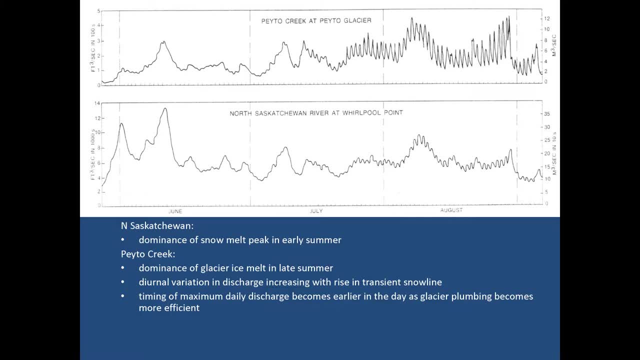 especially late in the summer. And if you were to look at the timing of the, the exact timing of the peaks, you'll find that as the summer goes on, the peaks become earlier and earlier. And that is because at the beginning of the season, 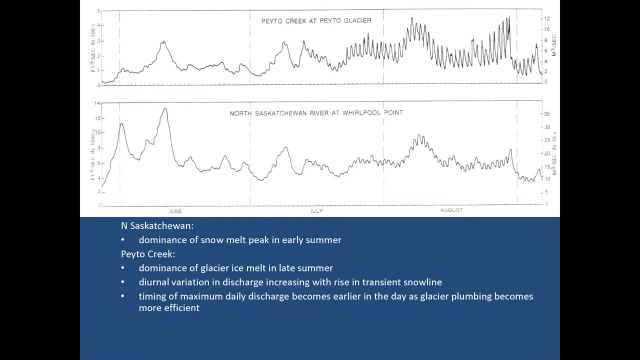 when the glacier ice has moved and filled up all the crevices and cracks and hollows, the water can't get through very quickly. But once melt water starts getting through and it wears away, if you like, the ice, the channels get bigger. 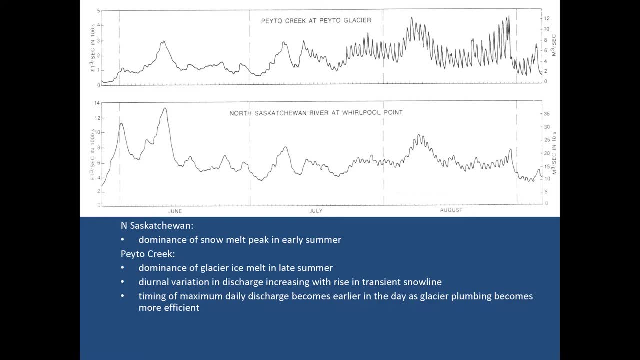 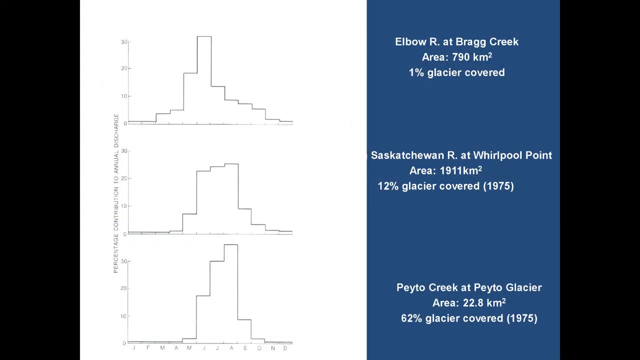 and the water can enter faster. So in fact, as you go on in the season, the daily peaks come earlier and earlier, And again on the top, a 1% glacier covered catchment. The timing of the peak: early in the season. 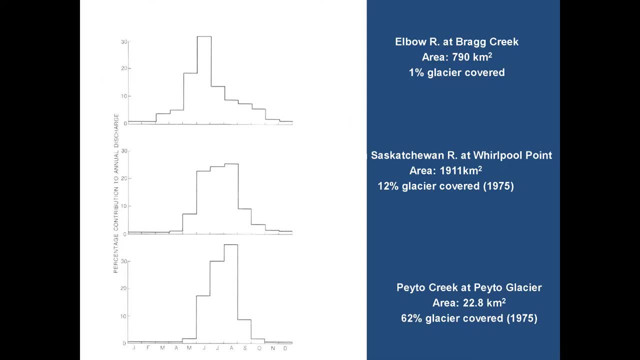 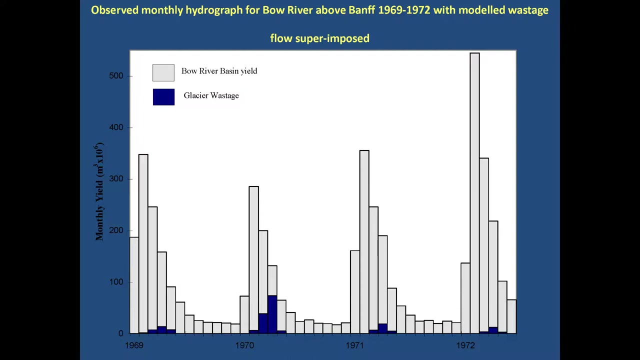 because it's snowmelt dominated At the bottom, a highly glacier covered catchment with much later peaks, And here again you'll see that. well, this is the Bow River at Banff. Quite big differences one year to another in the monthly discharge. 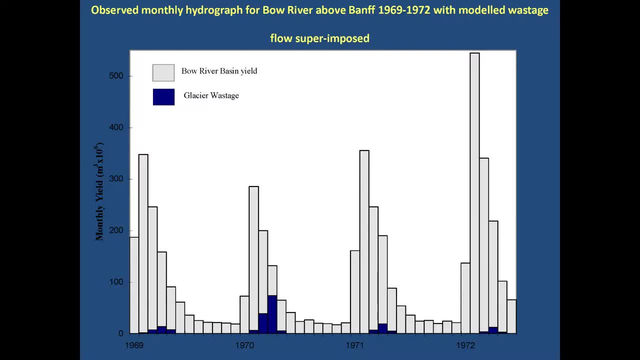 These are monthly figures. In 1970, there was very little snow, So the snowmelt peak is quite low compared to, say, 1970. So there was a lot more snow, But because there was very little snow, the glacier ice became there much earlier. 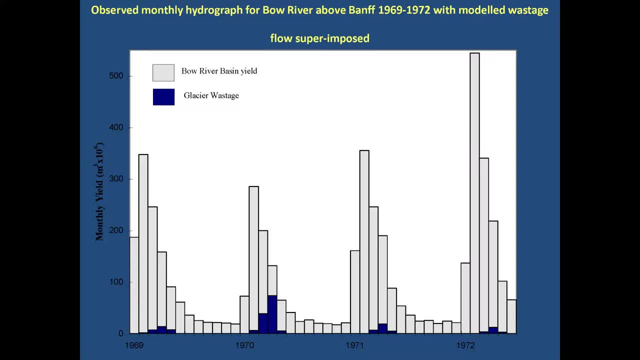 and ice melted. And here's the contribution of ice melt, Very large contribution relative to other years in a year when there's very little snow. So the glacier melt in fact compensates for low snow, Which is very important in the month of August. 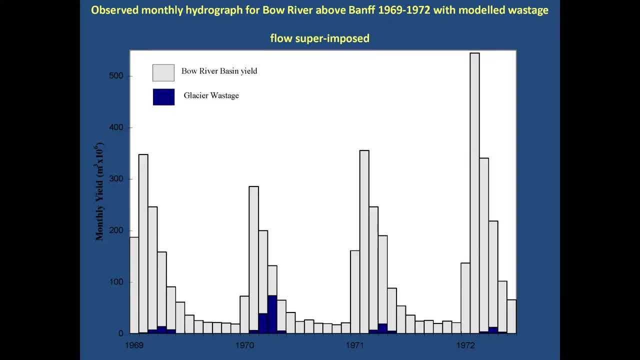 Half of the total flow in August for the Bow River at Banff comes from melting glacier ice. And again you can imagine, if the glaciers are getting smaller and smaller, that contribution is going to become less and less. So the buffering effect, the benefits of buffering. 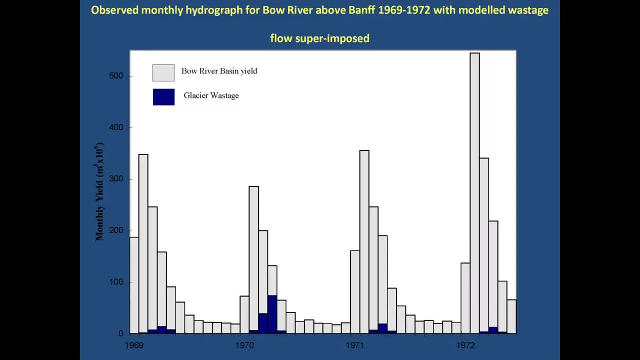 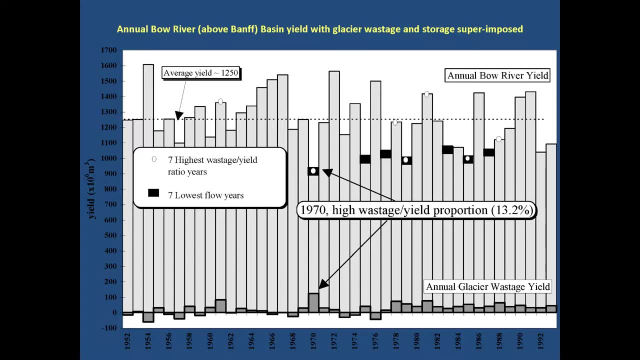 the benefits of glaciers are going to be less and less all through time And again. you can see this is the total flow at the Bow River at Banff And this is the glacier contribution down here. Sometimes there are positive, mostly there are positive. 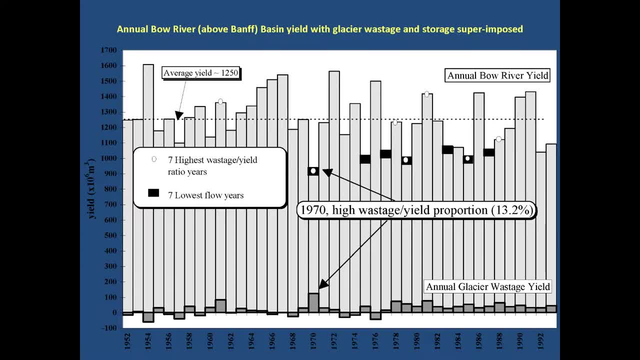 contributions of glacier ice melt. But there are some years when the glaciers, in fact, are growing. It's not every year that the glaciers are going to become smaller and smaller. Even now, the glacier can get a little bigger on some years. 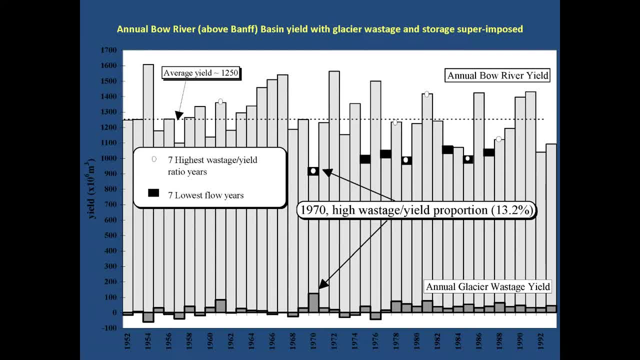 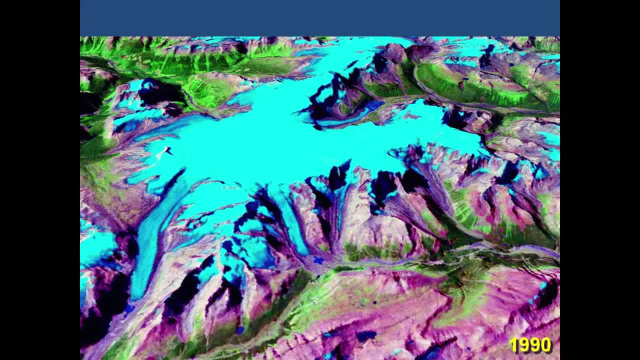 but it's unusual. And this is the Columbia Ice Fields 1990 and 2000.. This is the famous Athabasca Glacier here, the Saskatchewan Glacier, And just for that 10-year example, you can see how the glaciers have been retreating. 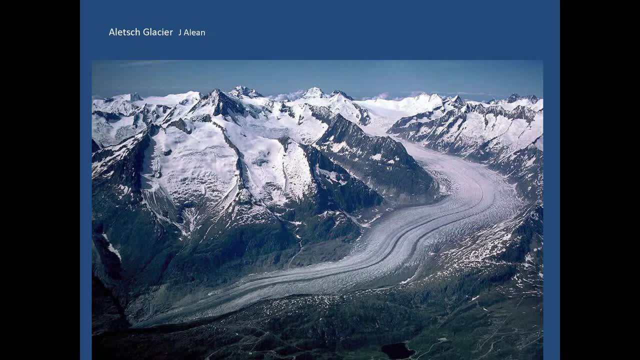 Well, now we're going to move to other parts of the world, And this is, in Switzerland, the largest glacier in the Alps, the Aletsch Glacier, And the waters from it and the surrounding hill slopes feed hydroelectric power stations, And I had an interesting experience here. 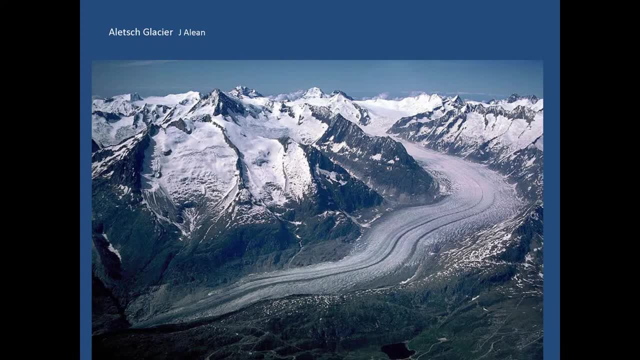 back in the early 70s, when I visited right up here on the Jungfrau fern, It was covered in pink. What was this? Well, it was dust from the Sahara, And it gets. occasionally it gets blown, covers the glaciers. 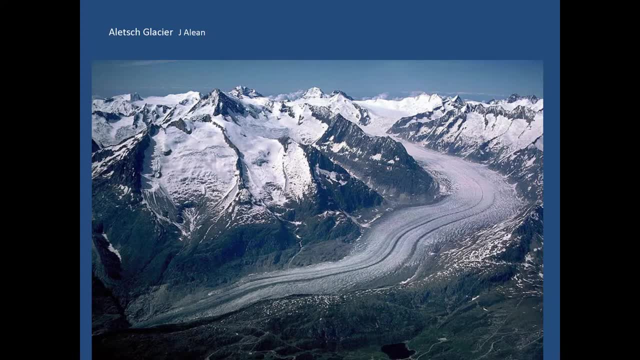 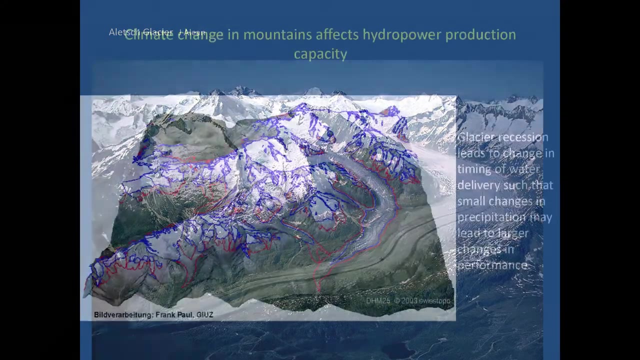 and greatly affects the albedo and contributes to melting, And in fact I think it was just in this. last year there's been a similar sort of Sirocco, a wind event from the Sahara, And again this is the same area. 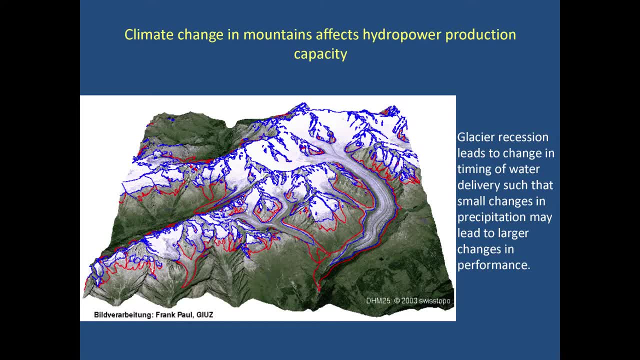 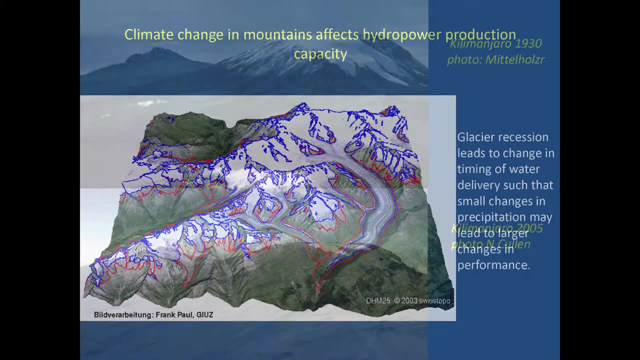 and it just shows how the glacier and its surrounding glaciers have retreated from And this affects the amount of water available and the timing of water availability for hydropower production. downstream Go briefly to Africa, So there's snows of Kilimanjaro. 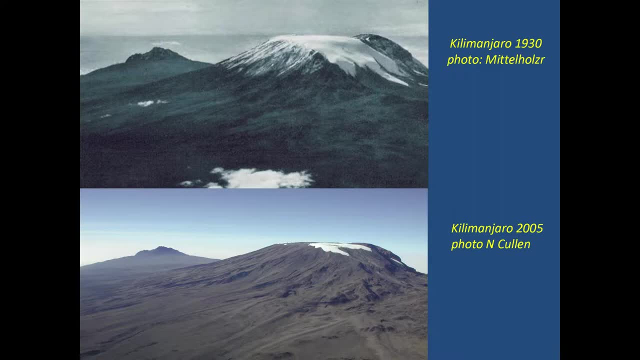 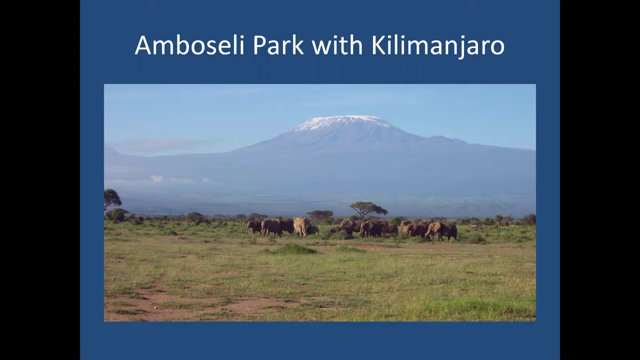 and a couple of pictures taken from pretty well the same aspect in 1930 and 2005.. And the big ice mass on the summit has been diminishing very greatly, With effects, of course, downstream. This is in Amuzele Park in Kenya. 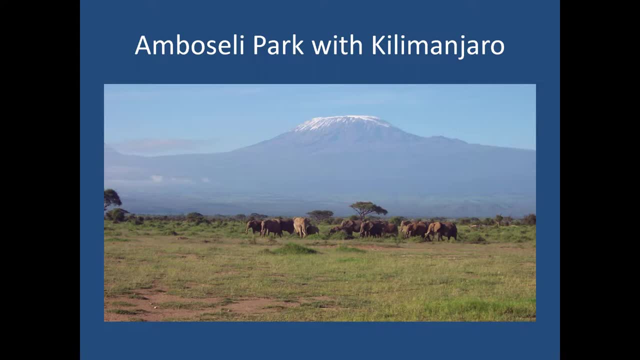 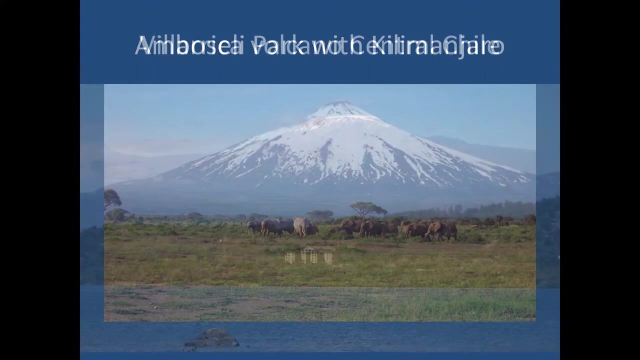 And the snows of Kilimanjaro not nearly so extensive and therefore not so much water given to the streams which come down onto the plains below and have effects on the whole ecological systems. So here is the cryosphere even in Africa having an effect on ecosystems. 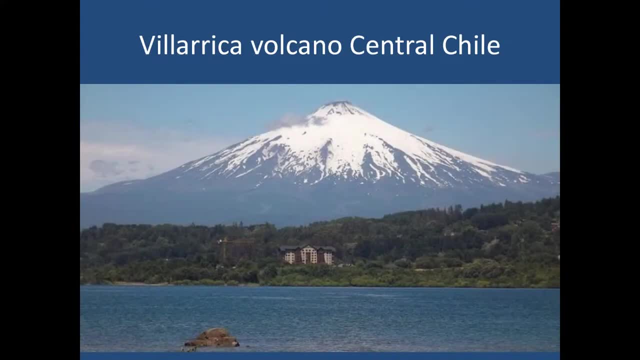 And take you just briefly. this is a volcano called Villarica in central Chile, which we visited in 1984.. And it was just before a major eruption. And here is the juxtaposition of fire and ice, because from our hotel we could actually see. 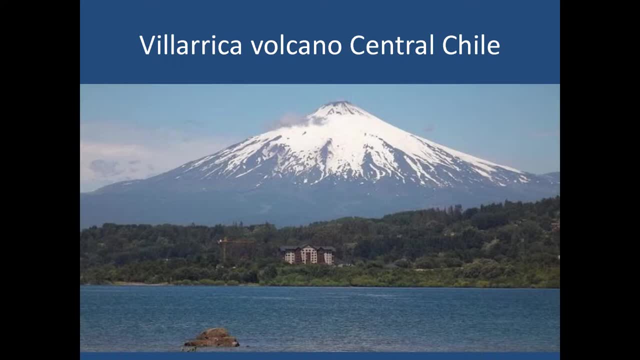 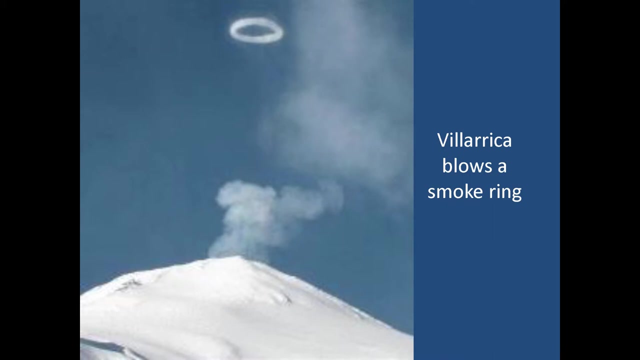 streams of red lava coming down through the glacier ice, And quite an interesting phenomenon was that it would blow smoke rings. It really does blow smoke rings And in fact I haven't got it in my collection of pictures, but we saw many smoke rings. 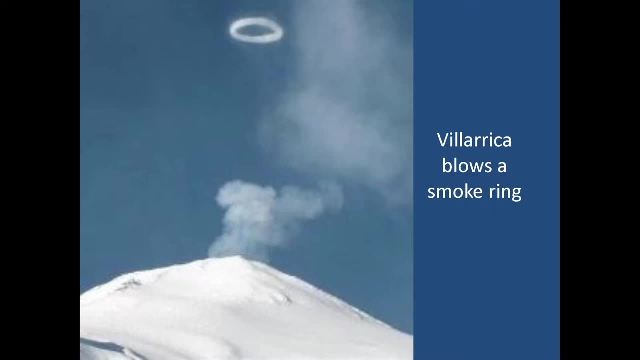 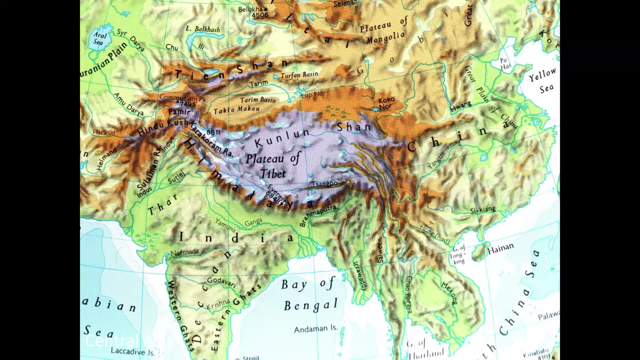 all at once in the sky. Well, we're coming to my second area of major work that I undertook in the Himalaya, but particularly in the Karakorum Mountains in northern Pakistan, in Kashmir. There there are the largest glaciers between 50 degrees north. 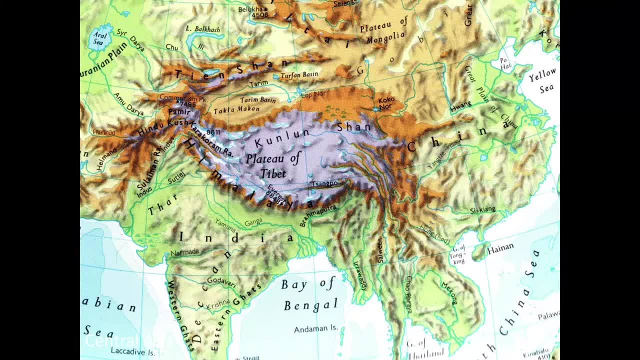 and 50 degrees south They are in fact, the glaciers of the Karakorum are, in fact, considerably larger than the glaciers in the rest of the Himalayan chain, And that's really because the Himalayas are a whole series of very steep peaks. 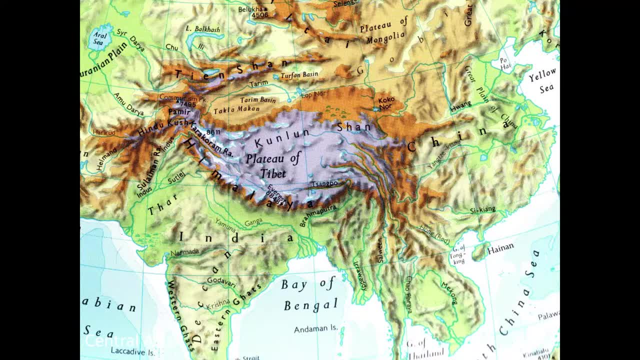 whereas in the Karakorum there's a great deal of land continuously at very high elevation and supporting, therefore able to support many more glaciers. Whereas in the Rockies and in western Canada, in mid-latitude situations, you get precipitation at all times of the year. 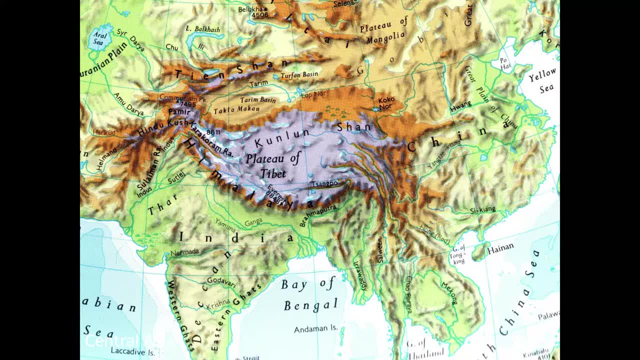 In winter, of course, it mainly falls as snow. in summer, it falls as rain, but there's no great seasonal difference. Well, that's very different in the Himalaya because, as you know, they have the monsoon, which comes in July through. 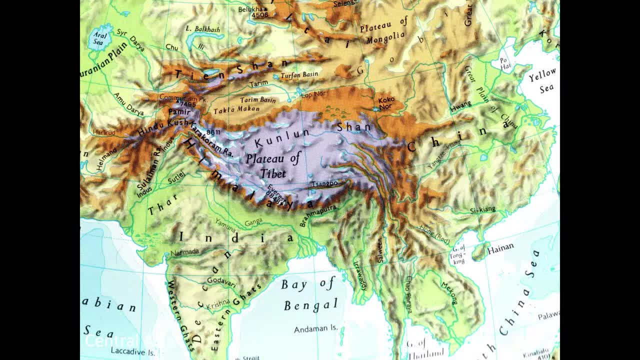 June or July through September, and the rest of the year is very, very dry, And so, funnily enough, that time of the year, in the summer, is the time where you have deluges of rainfall and, at the same time, 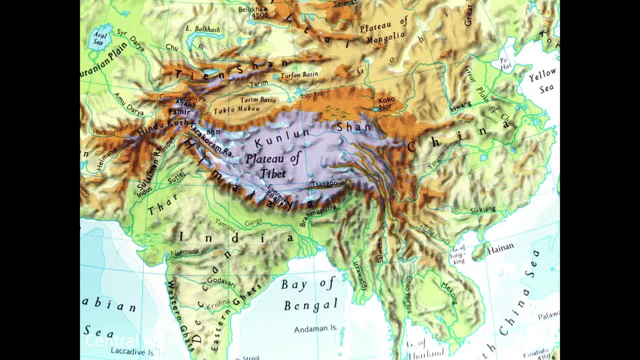 high up, you have accumulation of large amounts of snow, So the climatic situation is different. but it's different within this range too, because as you go westwards from this part of Sikkim and Bhutan westwards, so the monsoon becomes. 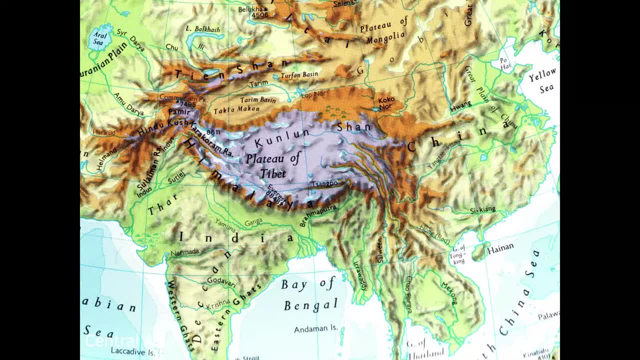 less and less dominant, and the Karakorum themselves in here are in fact shielded from most of the monsoon rains by this front range mountains like Nanga Parbat, and once you get into the Karakorum then there's a lot of winter snowfall. 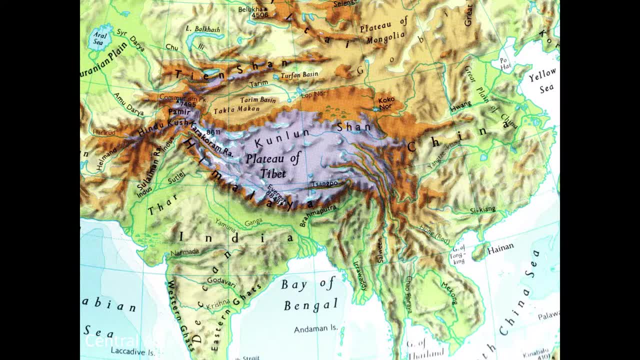 snowfall, which is derived from cyclones coming all the way across from the Atlantic. So the point I'm making is that the climate is not the same in all mountain areas of the world, and that has effects on the discharge of the rivers down the stream. 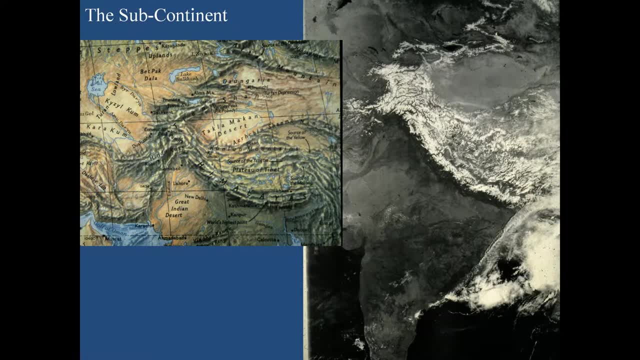 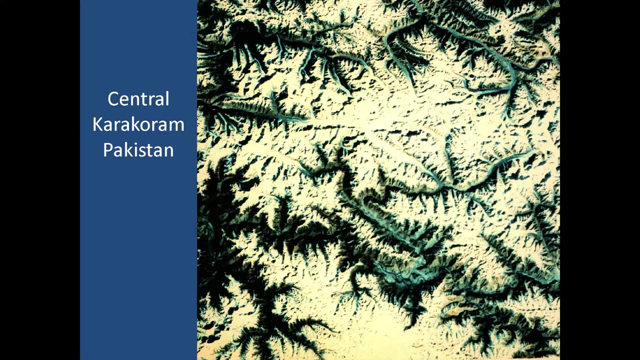 And here's just another depiction of that same area, the Karakorum up here, here, in the Himalaya, snow-covered, and this is the subcontinent down here, and here is the central Karakorum, and I'll just take you to. 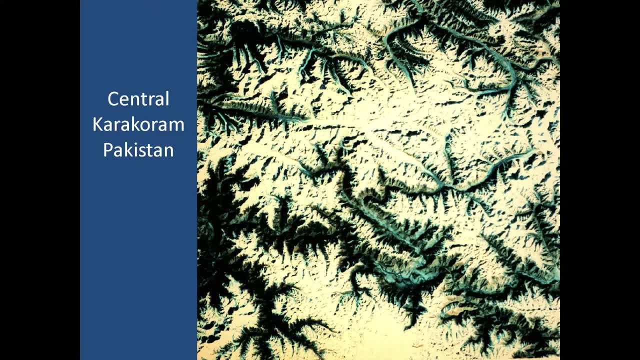 the Biafu Glacier, which was one of the glaciers that we studied: 560 square kilometres, much larger that glacier alone than, say, the Columbia Ice Fields, and about 60 kilometres of the valley, ranging from 2,500 metres elevation. 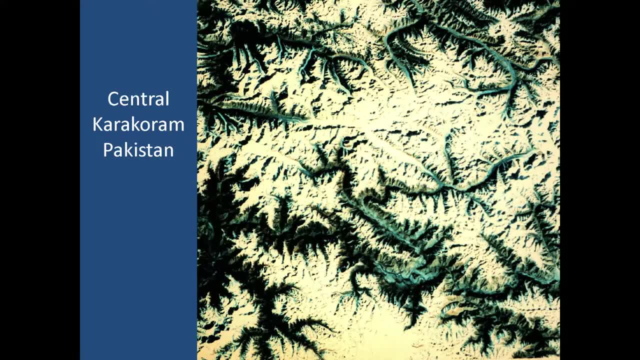 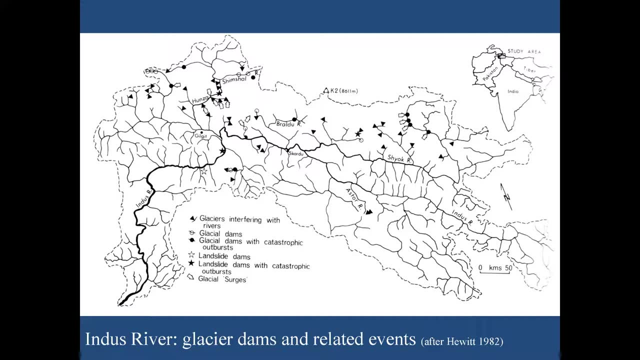 but once you get into the snow lake up here, you're up the mountains above 7,000 metres, And one of our good colleagues, Ken Hewitt at Wilfrid Laurier University, with whom I've worked extensively, has this is a map. 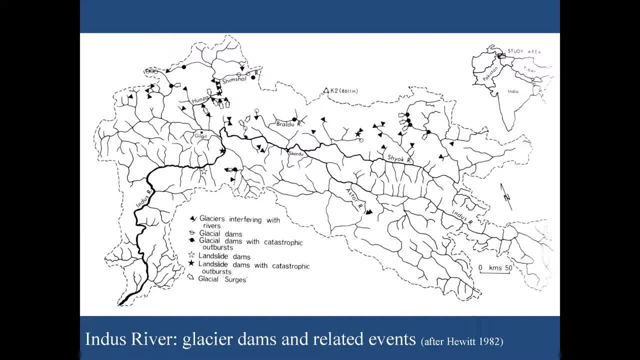 of his showing glacier-dammed lakes. Now in the Karakorum there are lots of glaciers which surge Every so often- every 10,, 20,, 30, 40 years, depending on the size of the glacier, the glacier will suddenly surge forward. 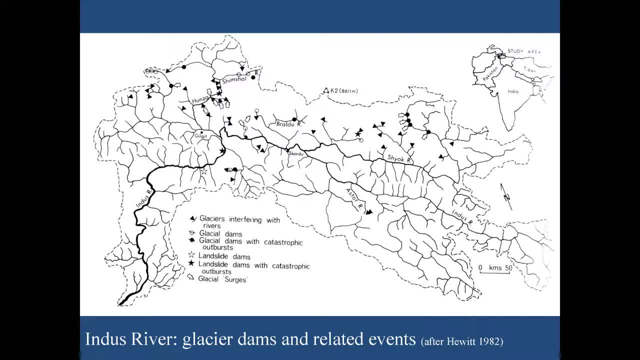 and sometimes run right across a valley and block it, and then the river flowing down that valley will form a lake behind and eventually the ice dam will break. Usually it's water going underneath the ice, the ice essentially floating on the water. 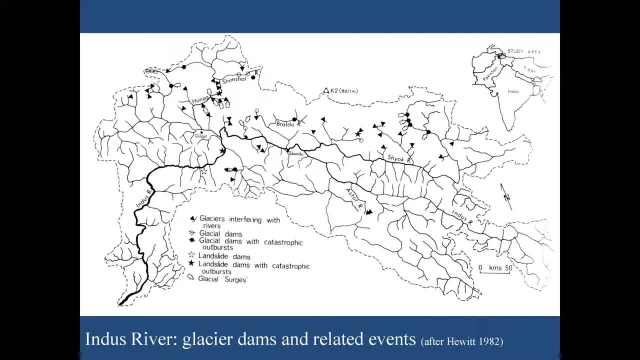 and that can initiate huge floods. And there was a case in two cases in the 1920s on the Shayok River way up here that there were two successive ice dam floods and the water took four days to travel down to Atok. 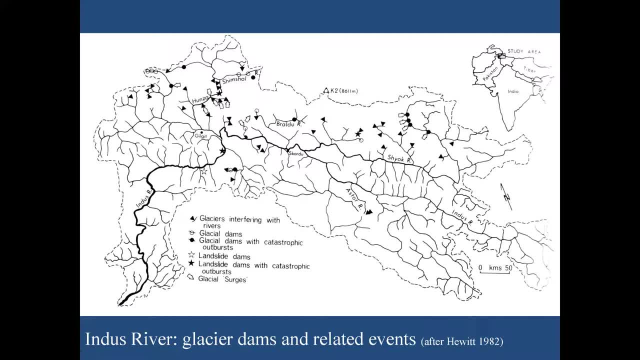 which is the where the mountain waters divulge onto the Tindus Plains. It took four days to come down, but even then the river stage- that is the height of the river, the height of the surface of the water- went up 18 meters. 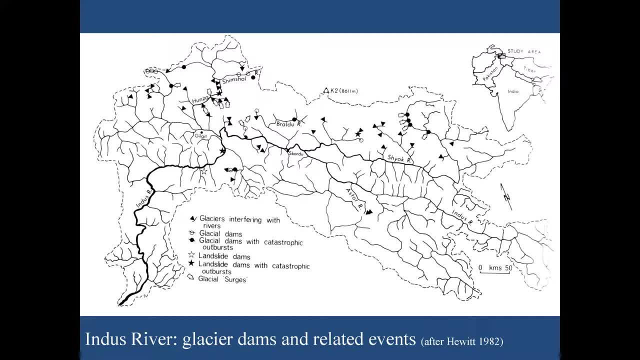 which is huge, And there was a case in 1841 of an army camped on the plains down below and they were washed away suddenly, because this can come really quickly And there are lots of examples of that. So the changes in the shape of glaciers, 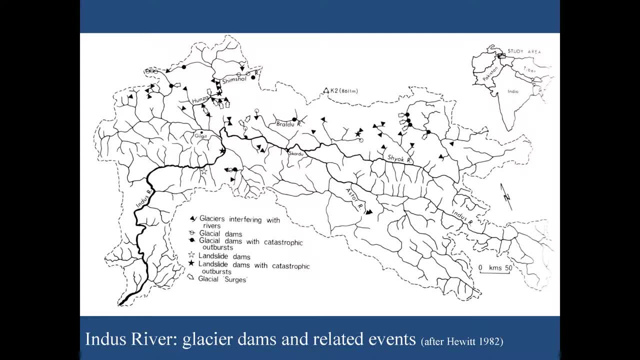 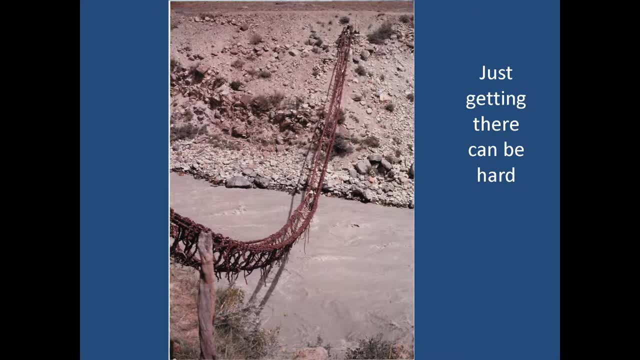 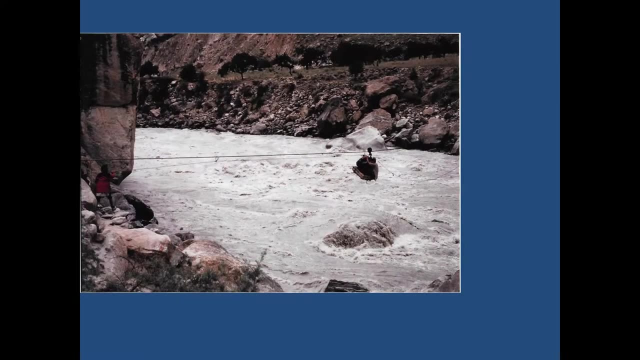 can really influence, in this case, the development of floods. Well, just a few pretty pictures of the difficulty of getting there to do field work. is somebody crossing on a rope bridge, and this is the way you sometimes have to cross rivers- being pulled across. 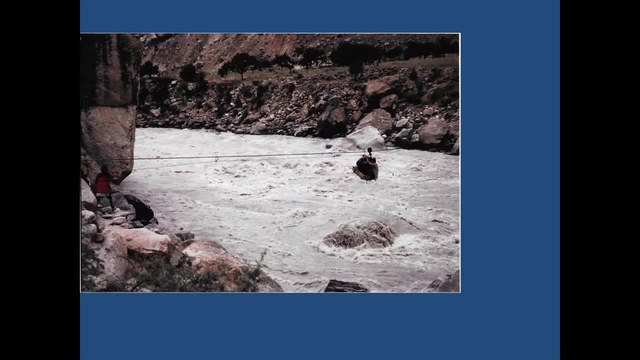 on these little trolley things And I made the mistake of grabbing onto the wire, and of course it takes all the skin off your hands if you're stupid enough to do that. And here we are walking up the Biafra Glacier. 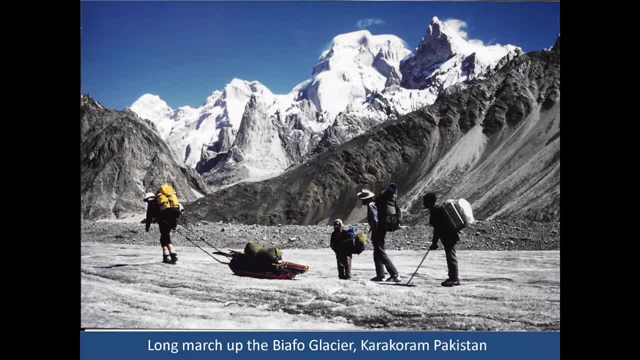 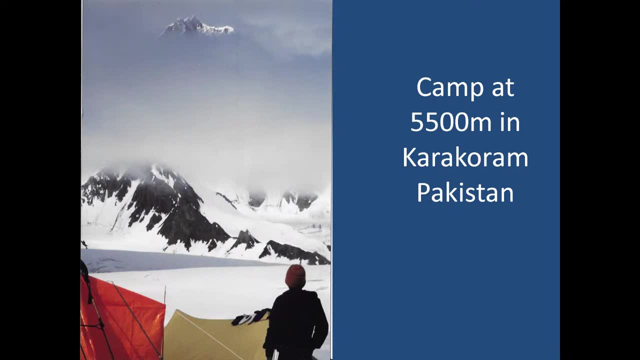 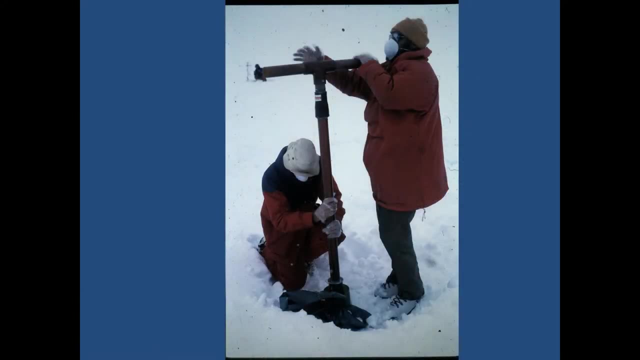 It took six days to walk up that first section And then we get into the snow fields at the top And in fact what we were interested in doing there was to take a snow course, because up at that high elevation, above about 5,000 meters, 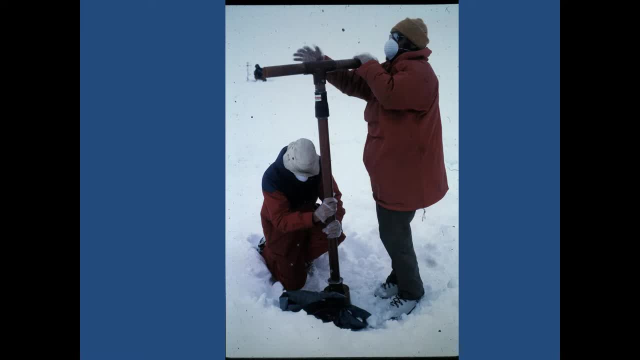 it's in the so-called dry snow zone. There's never any melt. Well, maybe there's going to be melt if the temperatures keep on rising, But it's the dry snow zone, and so each annual layer is well preserved And you can core down through those layers. 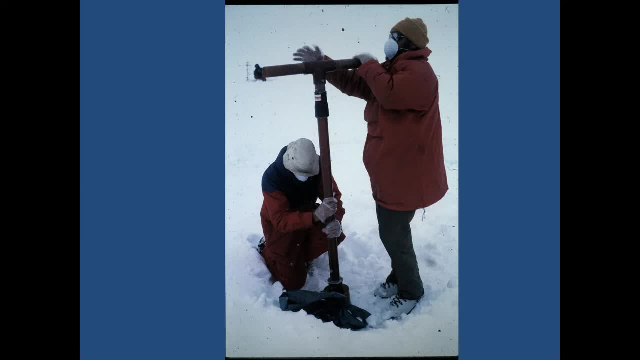 and you can say, okay, last year there was so much snow, the next year there was so much, the next year, and so on, And you can get a very good idea of the total precipitation up at that elevation And you may say: 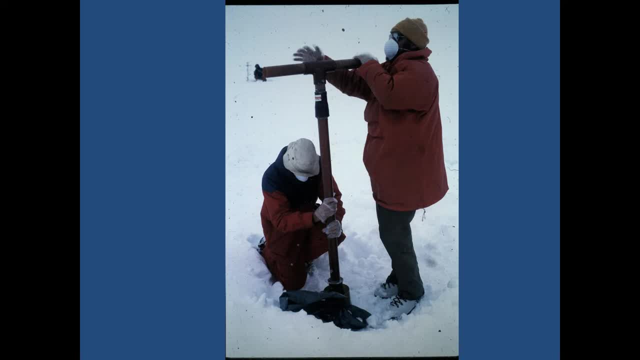 well, aren't there avalanches? Doesn't snow blow around and contaminate the records? Well, this snow zone up there is so large, 300 square kilometers- that you can go to places where there are no avalanches and the snow blowing in. 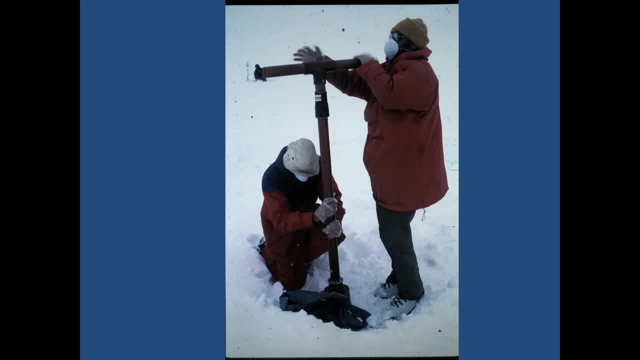 equals roughly the snow blowing out, And so you can get a very good idea of the accumulation of the precipitation at those high levels, And it is at the high levels that the precipitation occurs. Right down in the valleys it's very, very dry. 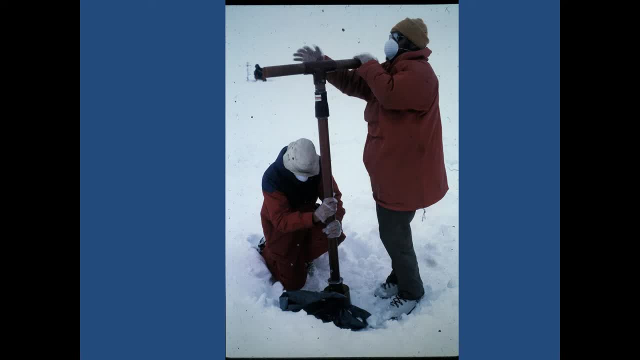 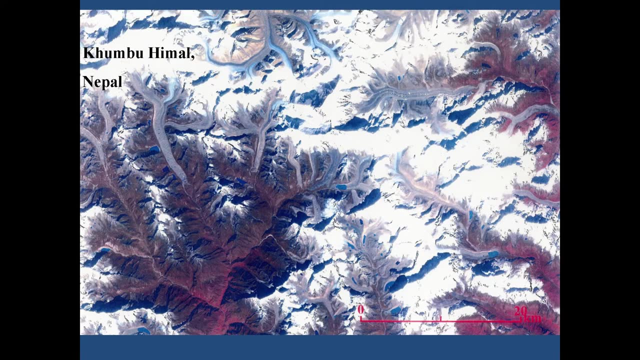 Virtually no precipitation. It's in the very high areas where precipitation doesn't occur, And I'll just take you to the Everest area. Everest is this, is the Khumbu Glacier here. Everest is in around here And you may be able to see. 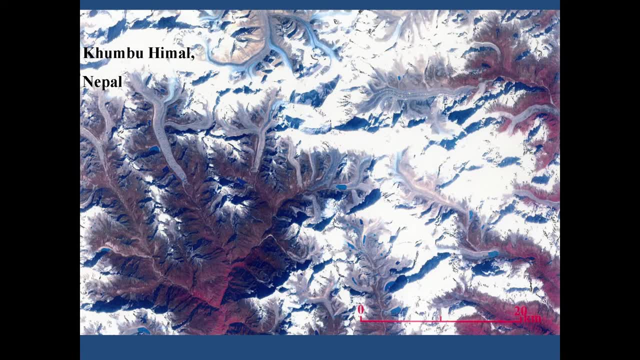 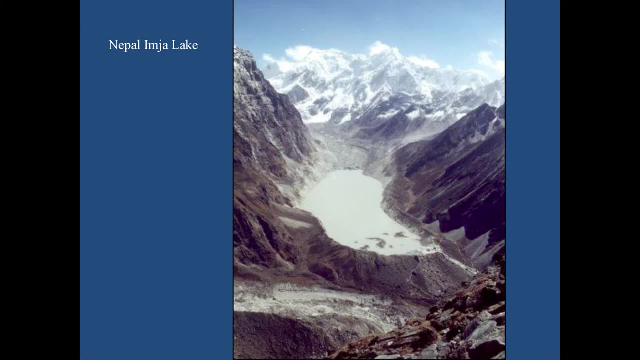 little blue places. These are little lakes. There's one there, There's one over here, And I'll show you that first one, the Inja Lake. These are lakes which are the result of glaciers retreating, melting, producing water. 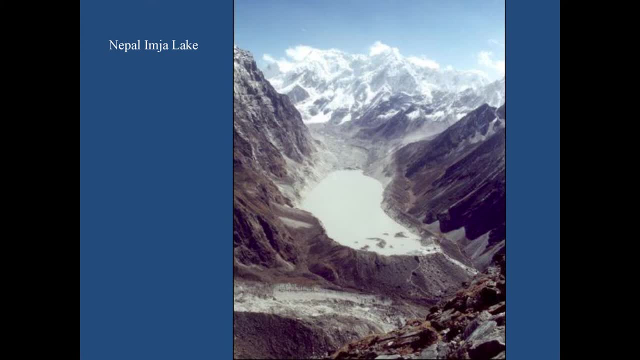 And the water is ponded back by the lateral and terminal moraines. And you can imagine that as the glacier retreats, as it melts, so those lakes are going to get larger. And you can also imagine that if there's a major landslide. 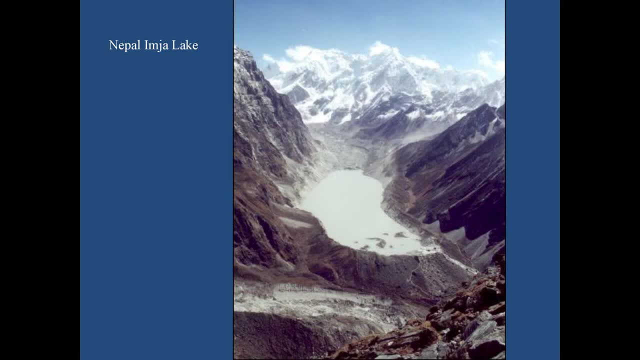 from these extremely steep slopes, the water will very suddenly be displaced And it will swap Down the valley below. these are called Glacier Lake Outburst Floods And they can be very short-lived, but very, very intense, And they're a real concern. 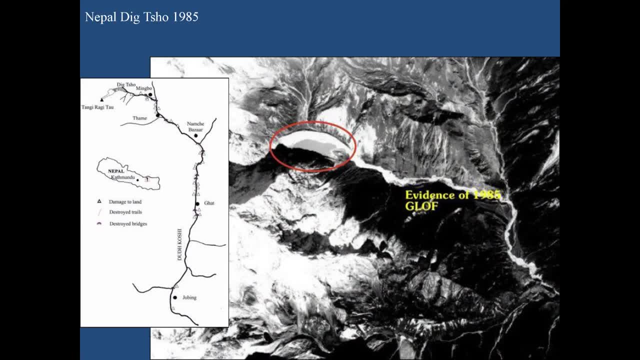 for many of the villages down below, And this is one such documented case called the Dig Cho. It's another little lake here. In 1985, it suddenly broke, loose Water swept down the valley And because it's such a lot of water, 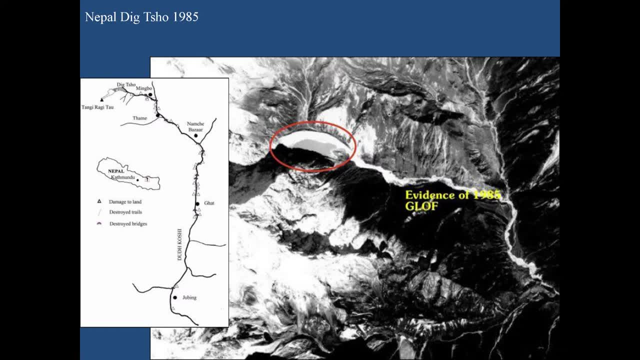 going down at once. it doesn't just go straight down the valley, but it slopes up this side and up that side as it goes down, And it can take out bridges which are 10, 20 meters above the water level, the normal water level. 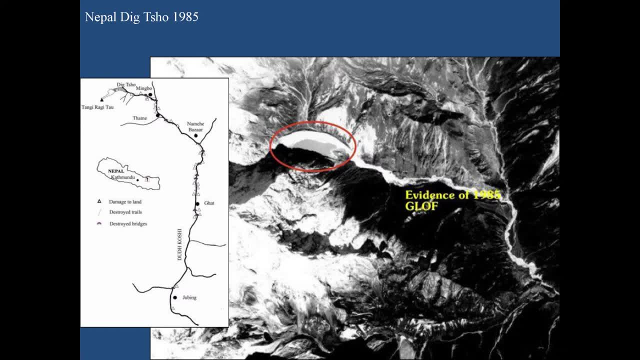 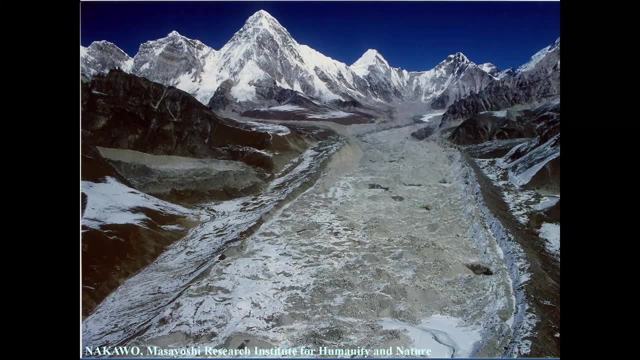 So this is an effect, a cryospheric effect on the lives of people. Oh, this is just the largest glacier in the Himalaya, the Nguzumpo Glacier, And we went up a small peak here at about 5,500 meters. 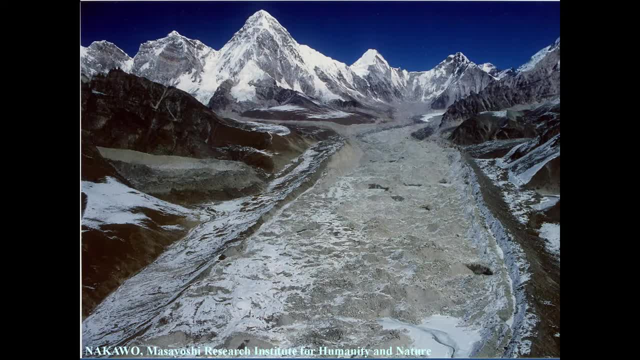 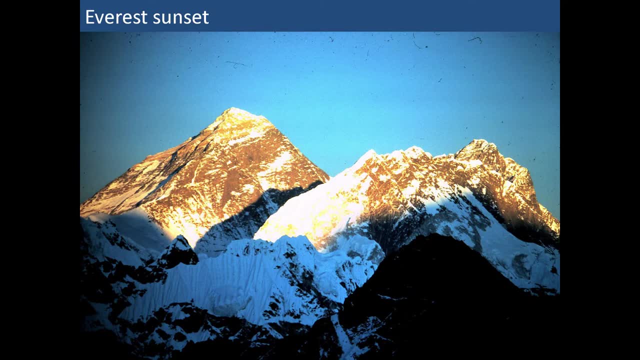 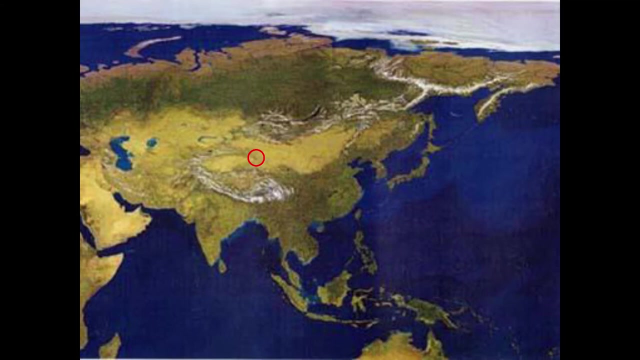 And from there you can see four of the highest mountains in the world And you get a very good view of Everest and Milt Sea and Lhotse in the evening sunset. Just one more example from Central Asia In the Kilian Mountains. 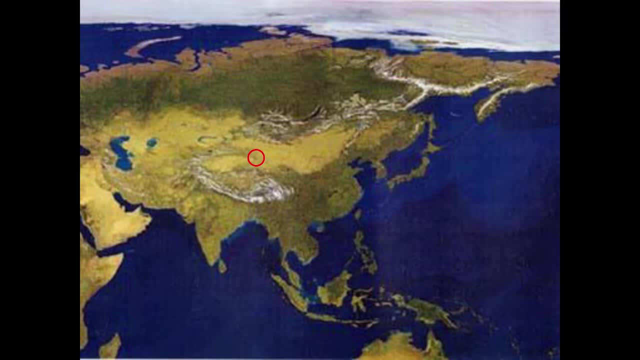 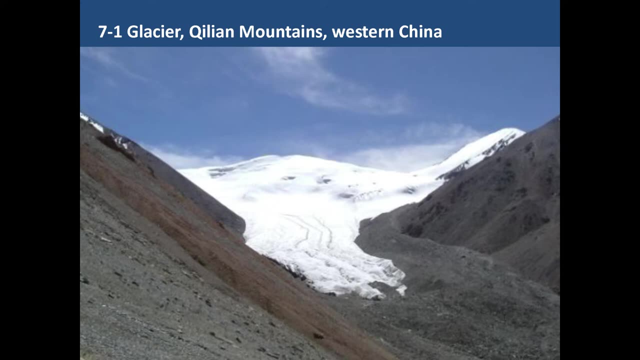 north of the Tibetan Plateau And here the glaciers in this mountain range has peaks of 6,000 meters, way higher than anything in the rest of Canada, And the glaciers here are also retreating, And in fact these are the mountains. 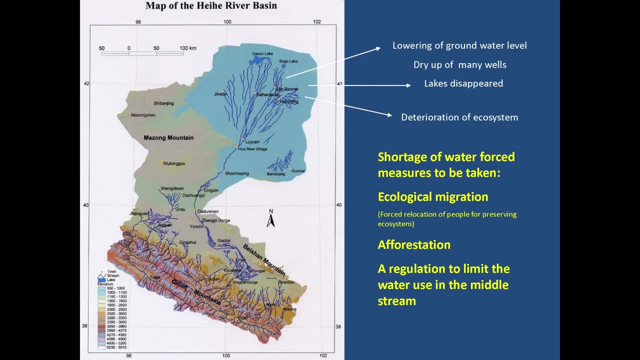 with the big river, the Haihe River, debauching onto the plains. This is the scale up here: 100 kilometers, And all these little towns or villages were part of the famous Silk Route connecting China to Persia in the far-distant past. 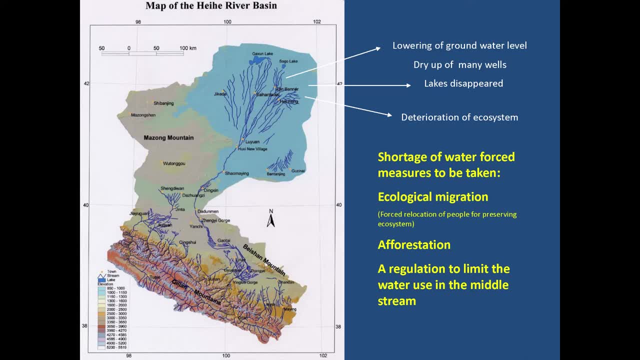 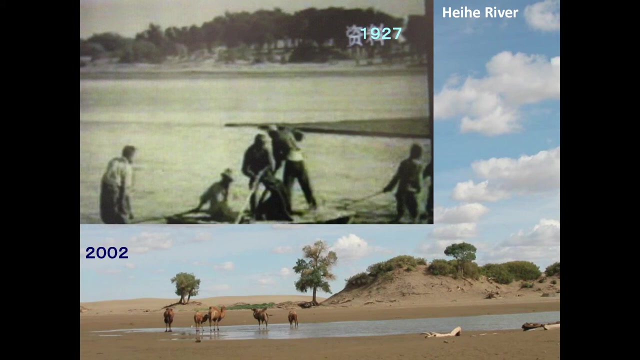 But the flow of that river has dramatically decreased, leading to more or less the disappearance of a huge lake and wetland area up there, 1927 versus 2002.. The 1927 picture is rather fuzzy but I think you can see. 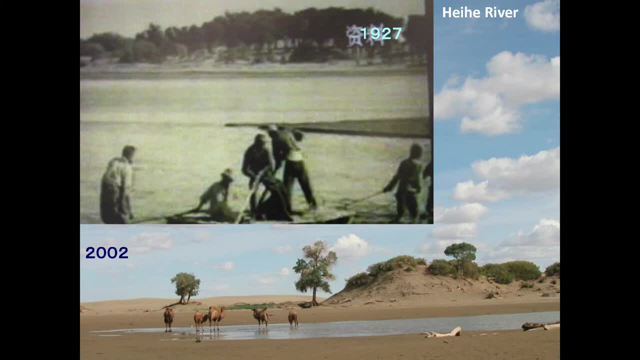 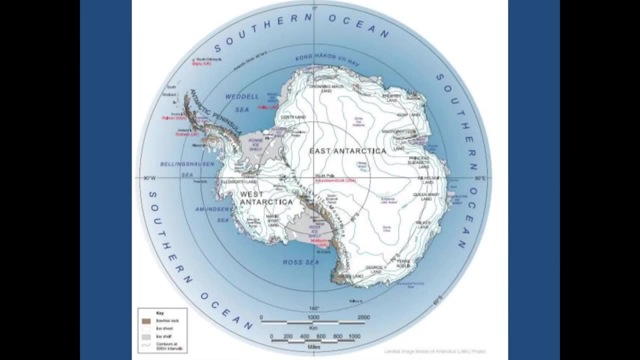 that there was a very large lake up there, and it's disappeared almost to nothing nowadays. Well, I'm going to finish by taking you to Antarctica, where, as I said, most of the ice in the world rests, and to the relatively small 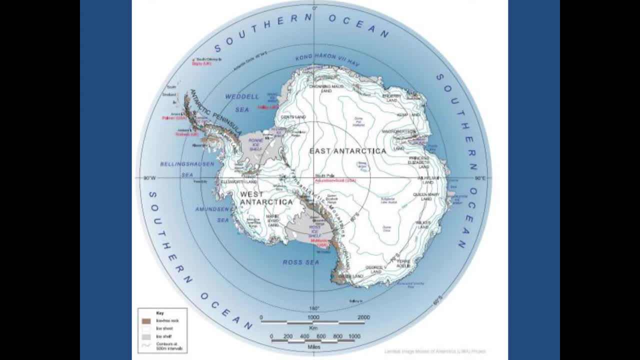 West Antarctic relatively small West Antarctic ice sheet compared to the East Antarctic. And of course there is, as you know, a great concern that if some of these ice shells which are floating on the sea, if they do break up, 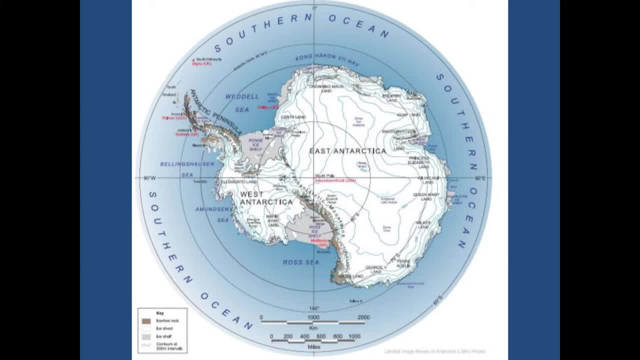 then they will release- take out the plug, if you like- from glaciers flowing into those areas And perhaps lead to instability and therefore a huge amount of ice going into the ocean and with a consequent rise in sea level. 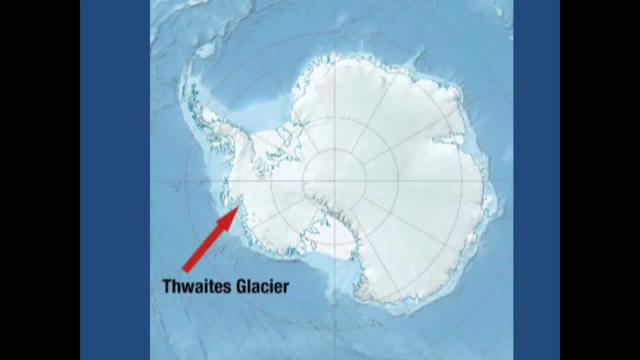 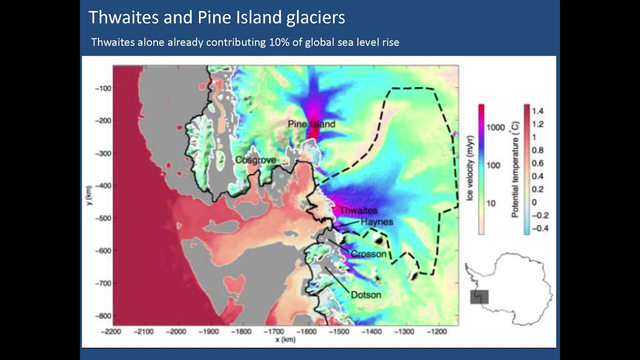 There's one particular glacier called the Thwaites Glacier, which is really an ice stream within the West Antarctic ice shelf. And, and here it is, This is the ice stream of the Thwaites Its. its front is about 125 kilometers long. 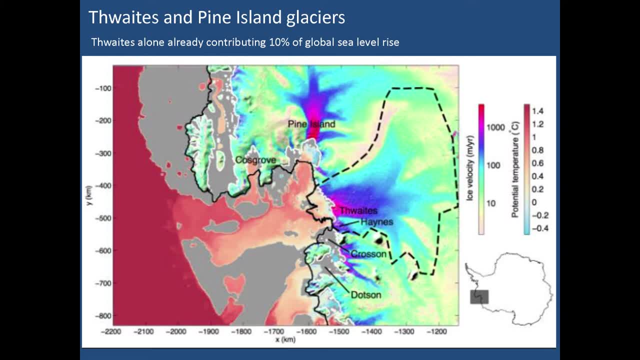 And it's going at in more than a kilometer a year into the sea And there's a. there's a similar but slightly smaller one up here at Pine Island And it is estimated. I'm really not sure how accurate this is. 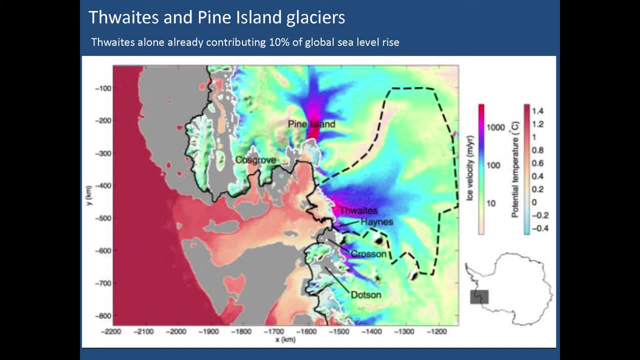 but it's estimated that the Thwaites Glacier alone is already contributing 10% of global sea level rise. As I say, I'm not sure whether that's true or not or how precise that is, but even if it's only approximately correct. 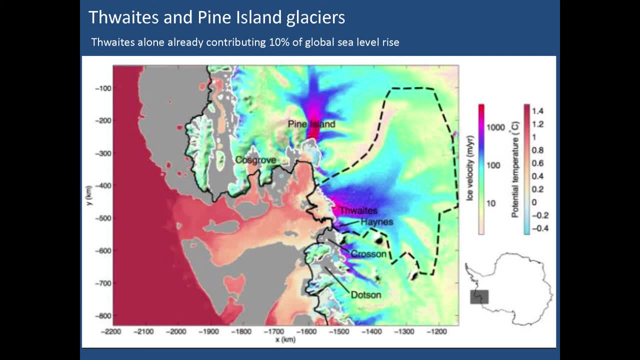 then that is really significant. If the Thwaites had completely melted, then it alone could raise sea level by about half a meter And, as you know, if the Greenland ice completely melts- which is unlikely in the next few hundred years, but possible- 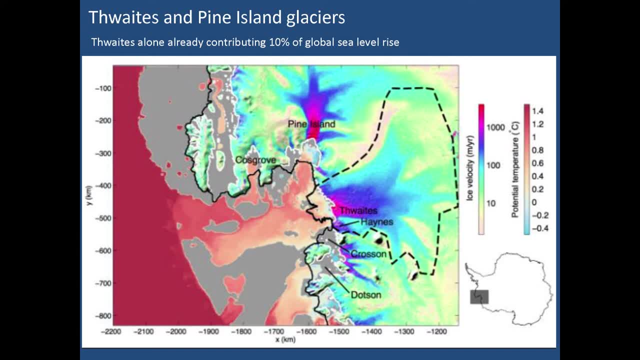 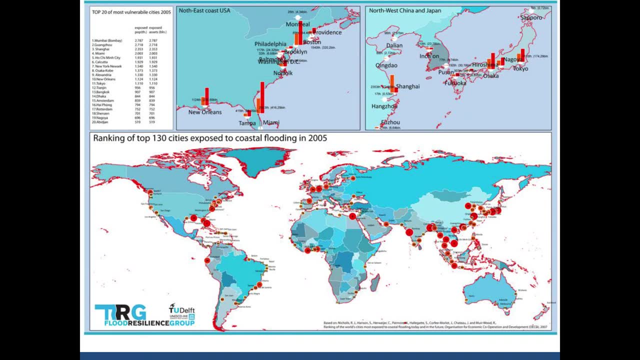 if that all melted, seven meters rise in sea level. And so we we should be concerned about those sorts of things, because many of the world's very large cities are right down at sea level And these economic and considerations have been developed. 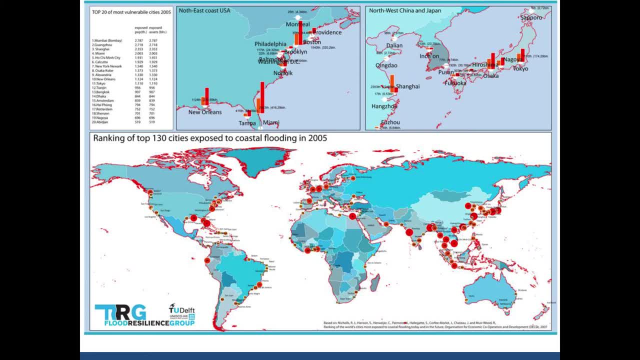 And they've listed here the 20 cities most at danger. And here's Mumbai And this. this is a few years ago that this was done, But anyway, nearly three million people would be displaced, with economic consequences of so many millions of. 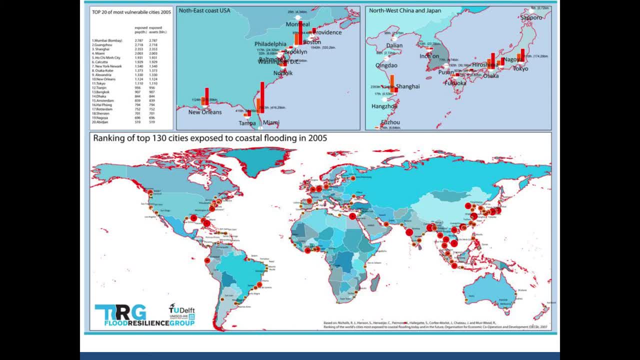 of you know dollars or the, whatever the financial unit is, And it's interesting, you see that Miami is number four in importance And yet Miami keeps on being developed, Which I don't know why. Well, I haven't covered.